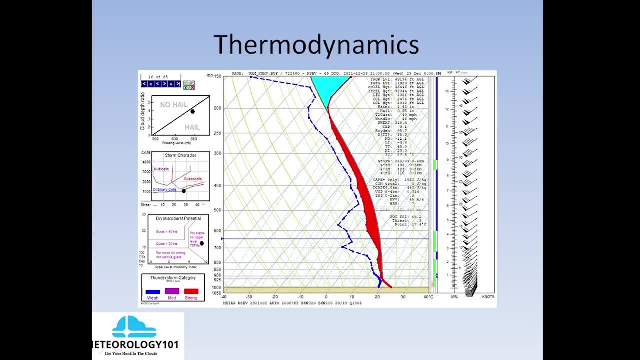 You can get all of the low, You can get all of your precipitation types off of these charts and how much of the air mass basically has modified when it's moved out of the source region. So if there's a continental polar air mass pushes down from the north, then how much moisture has it encountered? 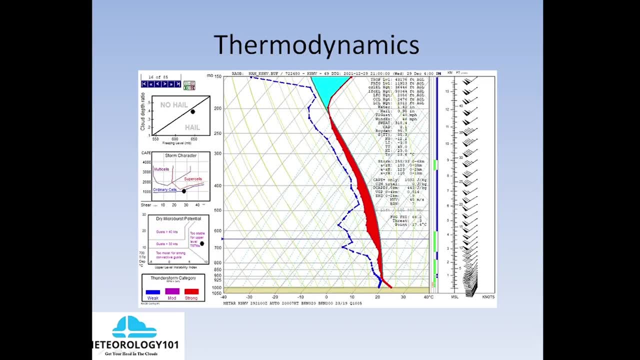 How much has it warmed from below? that modified that air mass as it pushes south And when these soundings are let go? it's every 12 hours, so there is a gap. but there are forecast models that develop these soundings And all that data is extrapolated onto these charts and then you can analyze these charts and pull up your energy levels, your cloud heights based on lifting an air parcel, cloud heights based on just heating an air parcel and causing it to rise. what level the cloud is going to form. 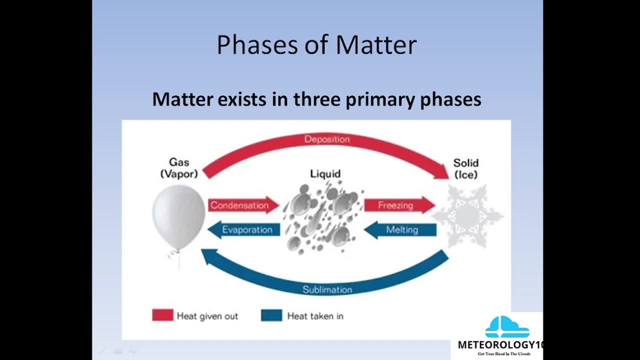 So there's a lot to these charts. So phases of matter. Matter exists in three primary phases. the phases the matter we're going to be focusing on- water for the atmosphere, solid liquid and gas- are the three phases so solid. in the solid state, molecules stay in a fixed state and have a low 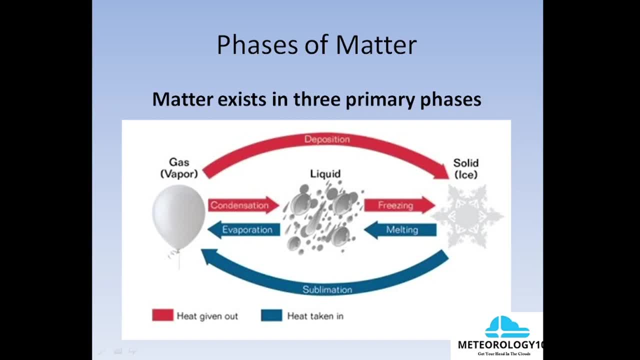 energy level. so think of it as: how fast are the molecules moving? as water is in each different state. if it's frozen, it's cold, it's not moving around much, so it's a low energy level. liquid state molecules move around, but they remain cohesive and maintain a constant density. 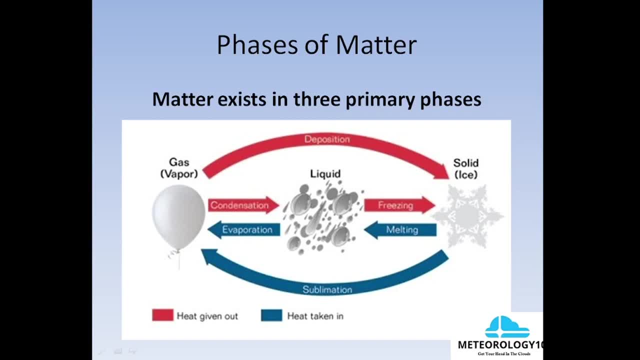 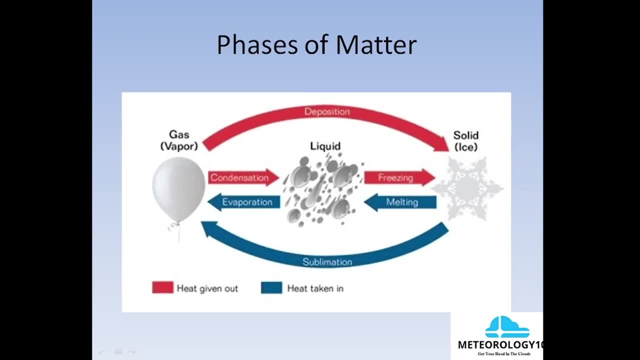 and then in the gaseous state, molecules are independent of one another and move in any direction and they have a very high energy level. okay, so in meteorology, what we talked about, we deal with phases of water. so solid is ice, liquid is water droplet, gas is water vapor. so in each 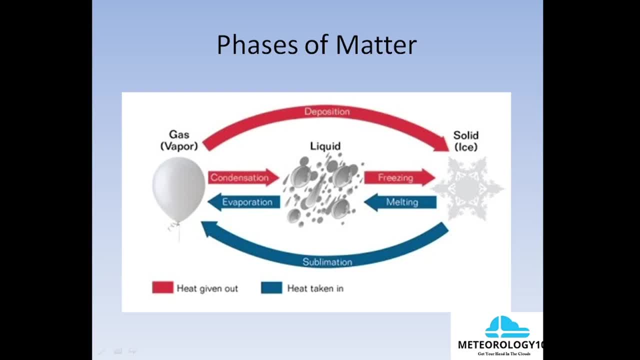 phase is favored at a specific temperature. so we know that the freezing or melting of water is 32 degrees celsius, or zero degrees, i'm sorry, 32 degrees fahrenheit or zero degrees celsius. boiling point of water is 100 degrees celsius or 212 degrees. 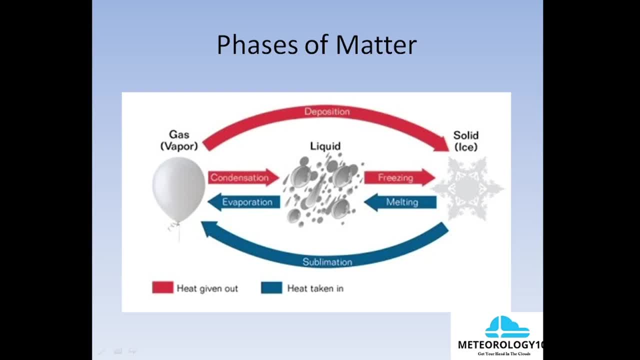 fahrenheit. so that is our mixing, melting and freezing levels and our evaporation condensation. so going back and forth now, um, the one we're most familiar with is going from a liquid to a solid. when the temperature falls, then we water starts to freeze, we get the ice on the ground, we get the snow, and then at what point? 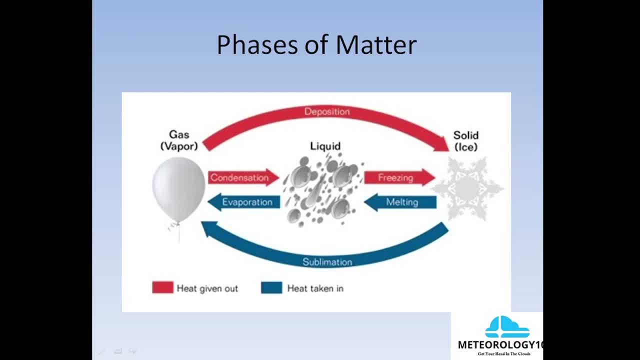 that the water is converted to ice. that is the most common phase that we think of. above that Ice is��고, awaiting its boiling point. that'll all this foundation at which of the cycles is reduced, are always taking place, and there's such a small portion of molecules that are knocked into a high energy state. they escape to a gas. so water does not have to be reaches boiling point to escape to a gas to become a vapor. so it doesn't have to hit that 212 degrees or 100 degrees celsius. it's going to change every so often. so while we have greatま Pottery, 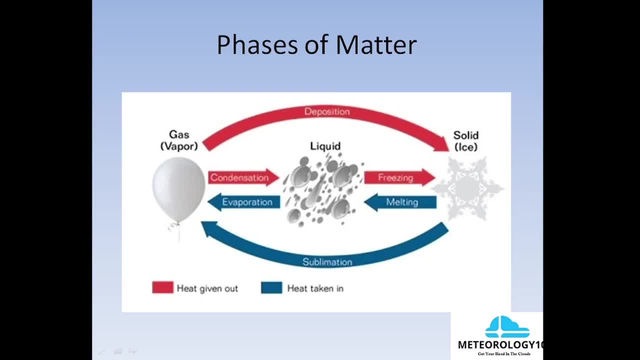 I just have a very- is to actually become a vapor, so you'll have steam- actually well before the boiling point of water, to ascend in a higher energy state, such as a liquid till gas. the molecules absorb energy. so think of when you're going from that solid state- ice- to liquid. you're absorbing heat, so the 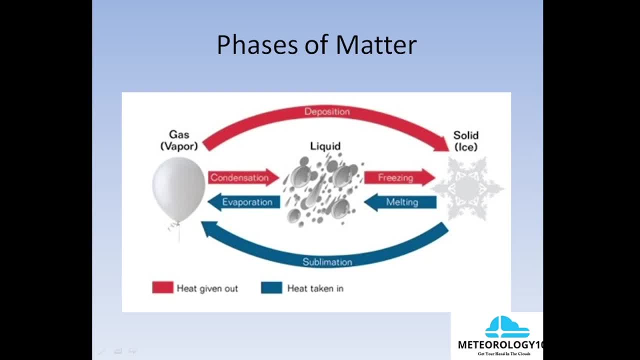 water droplet warms up, becomes a liquid, or the ice cube absorbs heat, becomes a liquid, and then that water droplet absorbs heat and then finally evaporates. so when descending to a lower energy state, then the release of energy is required by the molecule. so it's the opposite. when you got 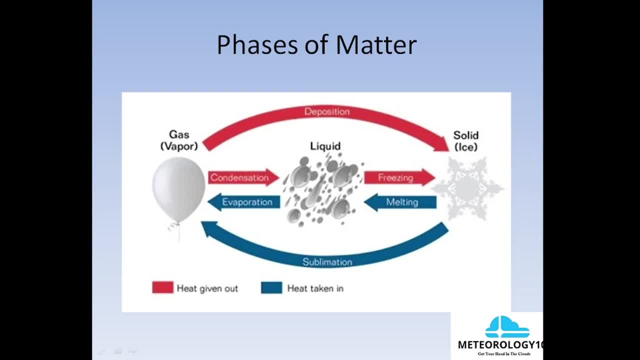 gas. you got a high energy state. molecules are bouncing off of each other. it's hot. once it starts to cool, those molecules slow down. so it reaches a lower energy state to become a liquid. then it be. then it starts to become, starts to condensate into a liquid, but like just remember, in clouds, you have to have something for. 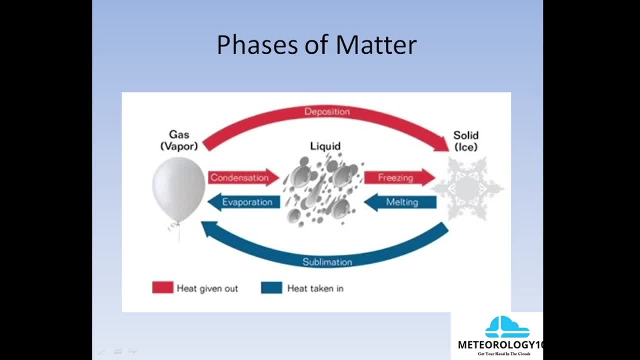 that water to condensate to, and that is the release of latent heat in meteorology. when it releases that heat from a gas to a liquid, it's releasing heat so that heat goes into the atmosphere and actually warms that air mass. so that's when we talk about the air mass moving. 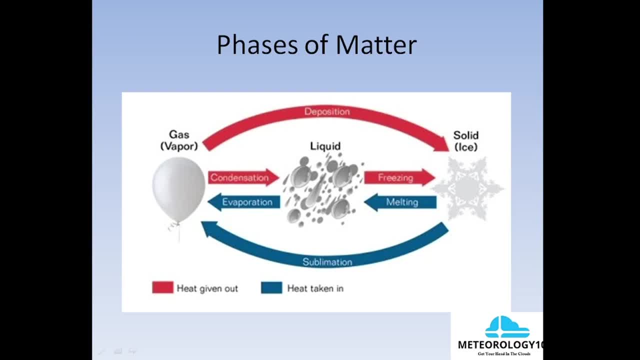 over a cold polar air mass moving out of the north, pushing south. it's moving over that warmer air and then that warm air getting absorbed into the colder air and creating a higher energy state there, but actually heating from below. so it will modify that air mass. so the release of latent heat, very important in meteorology when you think of water. 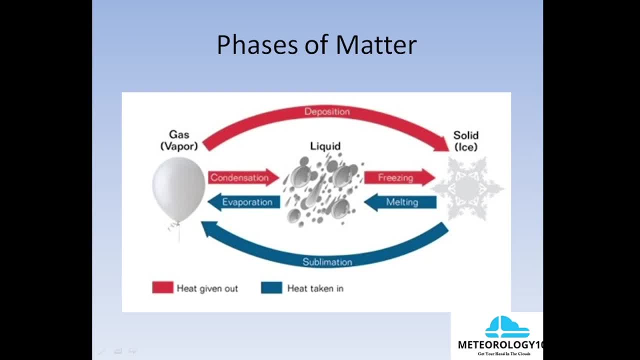 it's actually raining. if you ever seen it rain and evaporated before it hits the ground- that is virga- then that energy is released into the air around it. it actually will. evaporation is a cooling process, so it will actually cool that air mass. and that's these. 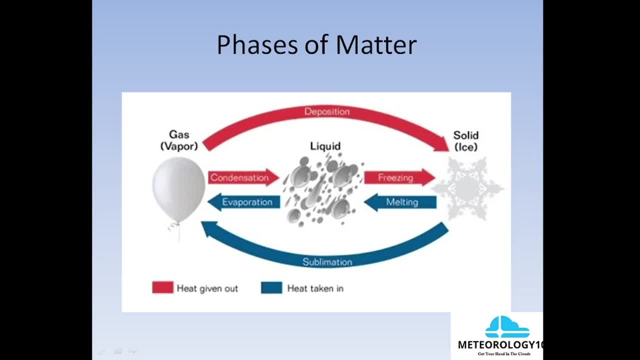 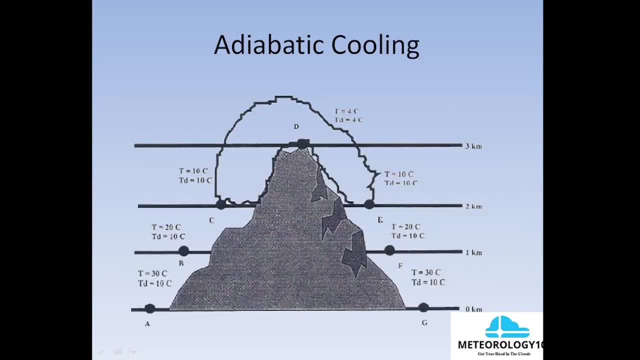 processes are what's mainly responsible for heating or cooling weather systems within our area. okay, so when we talk about lifting an air parcel or forcing an air parcel down, there are several times it lifts: frontal lift or graphic lift, heating. so when we force an air parcel up like: uh, the 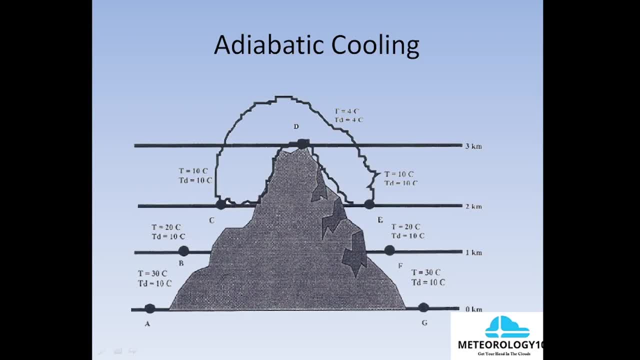 horror graphic lift in this picture. when we start to force that air that up we go, it's a dry air parcel. it's not raining, not rain being forced up the mountain, it's air so that contains water vapor, but it's pushed up. the temperature of that air partial starts to cool. 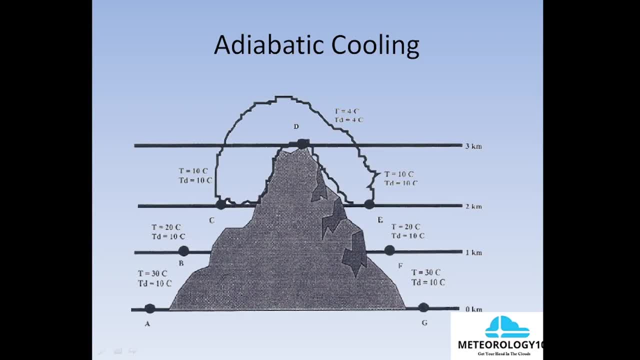 and it will cool at 10 degrees celsius every uh 1 000 kilometers, so as the air partial rises, it can, then it will. eventually the temperature will drop to the dew point and cause condensation, and then that's the level at which the clouds will form. so when we talk about their scooties, 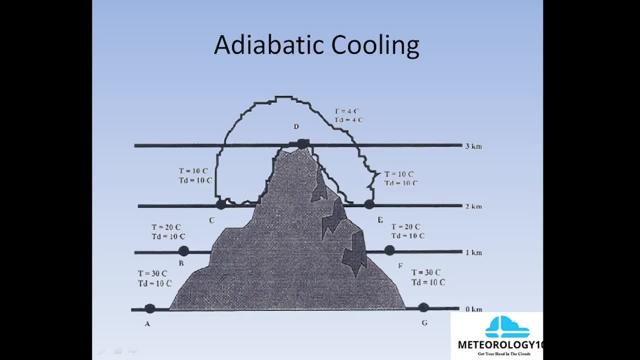 the lifting condensation level, the convective condensation level. how an air parcel is forced up depends on where a cloud layer will form. so the air parcel rises, expands, cools the molecule, take a lower energy state, achieve a lower energy state and the rating cooling is given by the dry. 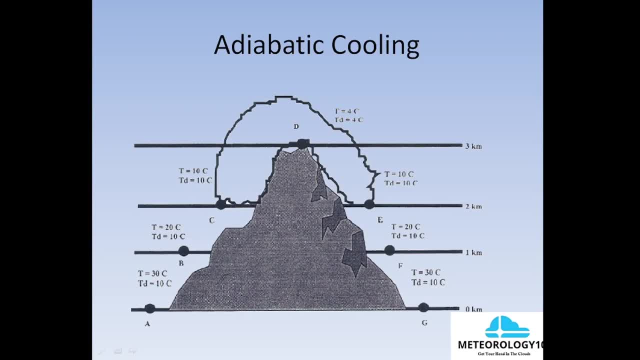 dry adiabatic lapse rate until it reaches condensation. once it reaches condensation, then you have to rise that air parcel moist adiabatically after that, and that's a different temperature because, remember, you're um warming that atmosphere by it cooling, but releasing the 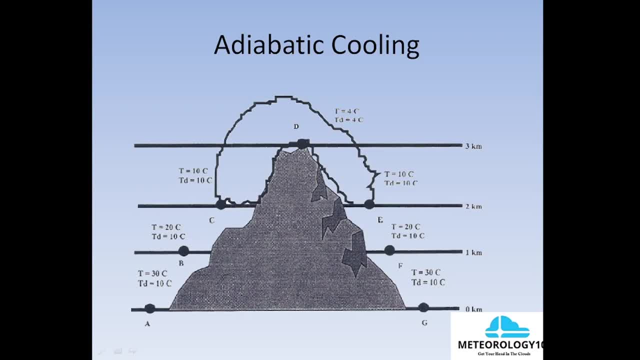 latent heat, so it's heating the air around it. so now it's approximately four degrees celsius difference on that. so as we go up in the pushing forcing this air mass, this air parcel up the mountain, we're dropping 10 degrees every thousand kilometers, or every one kilometer would be a thousand meters. every one kilometer, 10 degrees until. 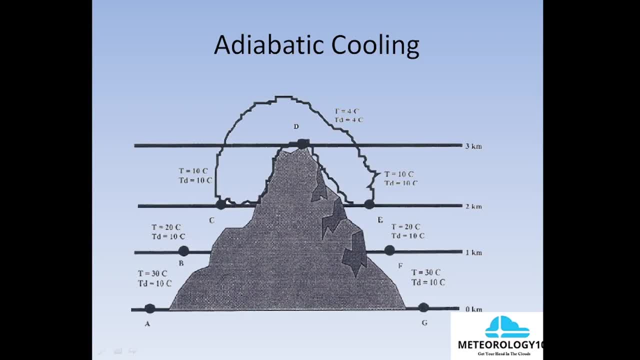 the temperature reaches the dew point and condensation occurs, and then it's going to drop six degrees every thousand kilometers. after that, once that air parcel gets over the mountain and starts to descend, then you're going to go moist adiabatically until saturation, until the water evaporates, and then so it's going to be back to the four degrees. 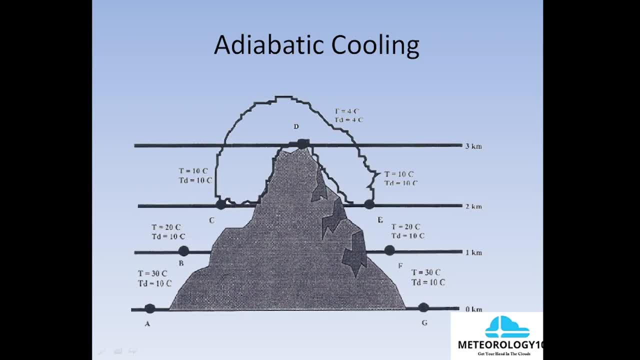 and what you end up with is 10 degrees every thousand kilometers after that, and then you'll end up basically at the same temperature you started with when you started to rise. so the air parcel will go through that complete process and end up right back where it started. 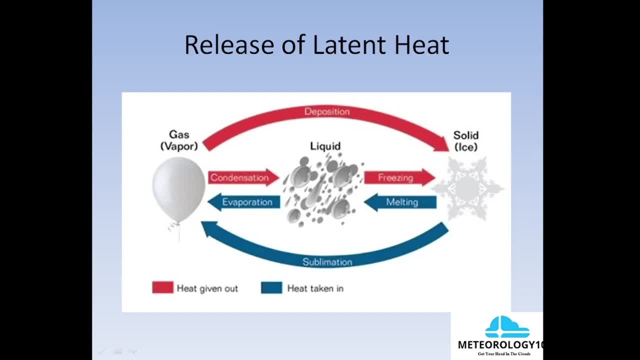 okay, so release of latent heat. um, if an air parcel cools to its dew point, then it achieves saturation. we just talked about that. a cloud forms. any further lifting will cause condensation in the form of water droplets or ice crystals. so once you reach the the point of saturation, then it has to, like i said it has. 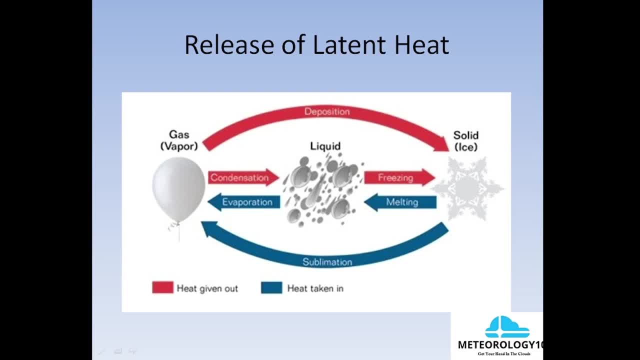 to have something dirt, salt, dust, something to condense to in the atmosphere, and then that's when the water droplet forms, or the ice crystal, depending if you're above the freezing level or not. then you have an ice crystal, say a cirrus cloud, 20 000 feet up. you're pretty much always above the freezing level. 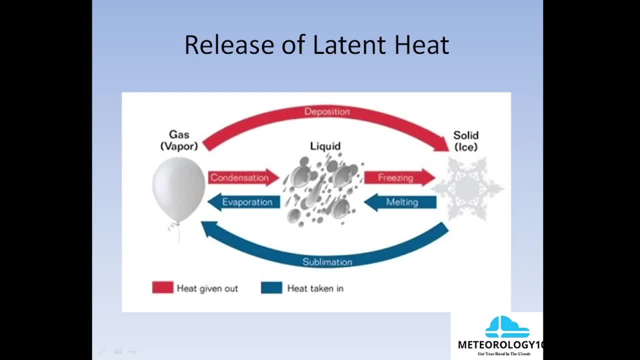 then you'll have ice, a cloud made of ice crystals. anything below the freezing level you'll have a cloud made up of water droplets. so the phase change, by its very nature, releases latent heat. so you're cooling, so you're releasing heat, so you have to be releasing heat to cool now. 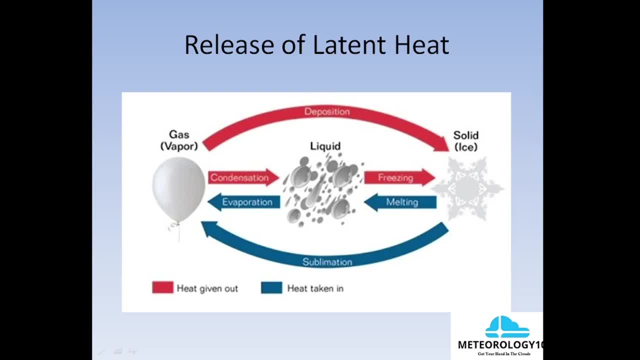 the heat is released into the air parcel and the air parcel begins to warm again. so once that condensation takes place, you're releasing latent heat. now, the air parcel itself, that column of air, an air parcel, is just an imaginary cube of air that meteorologists use. 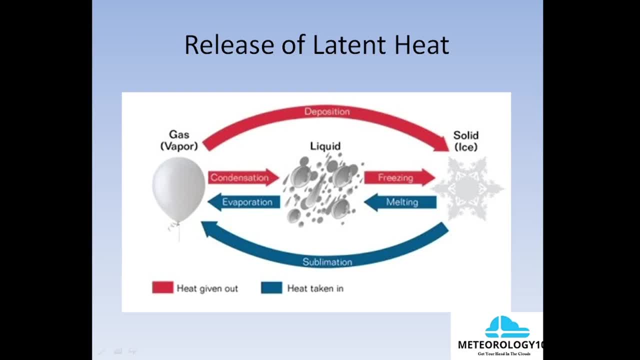 to put things into perspective. so it's not like any certain measure of how much air you know is this is happening with. it just depends on. it's just. this is just to project the image of, okay, an imaginary cube of air rises, cools, condenses and releases. releases that latent. 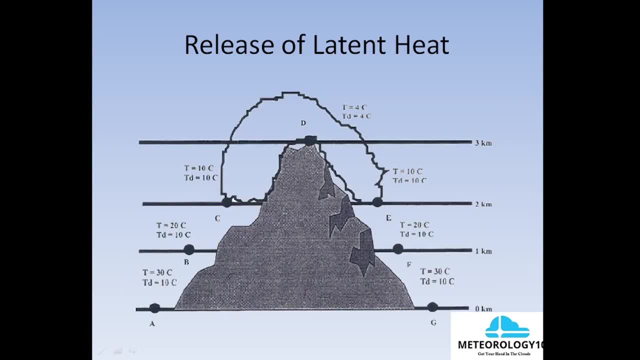 heat. all right, so back to that chart that we were at a partial which is lifted, one kilometer will be 10 degrees warmer from the release. release of latent heat, overall cooling rates from 10 dg to six degrees per kilometer once, like, like i said, once it reaches uh. 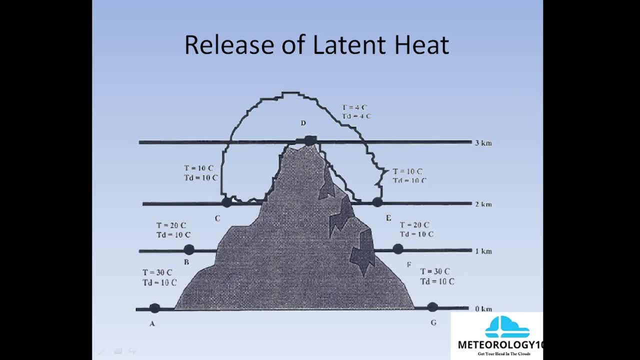 saturation. once that temperature drops to the dew point, then that heat has been released. now you're got a four degrees difference on a moist adiabatic lapse rate than you do the dry adiabatic lapse rate. so as lifting continues higher into the trope of troposphere, less and less latent. 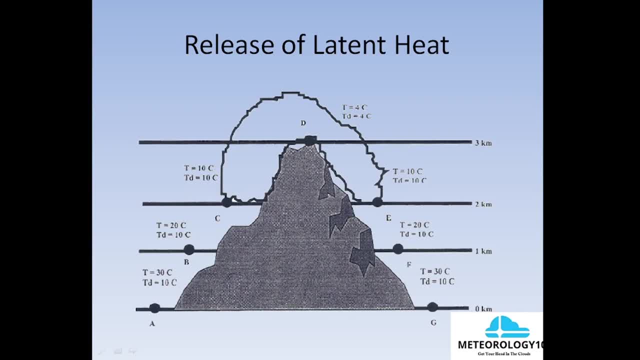 heat is released due to the dwindling amounts of moisture in the parcel. so you're running out of that moisture as that heat is released. the actual moist adiabatic lap rate- lapse rate- becomes much larger at that point. so how does this affect the weather? let's get into that. um, let's cover. 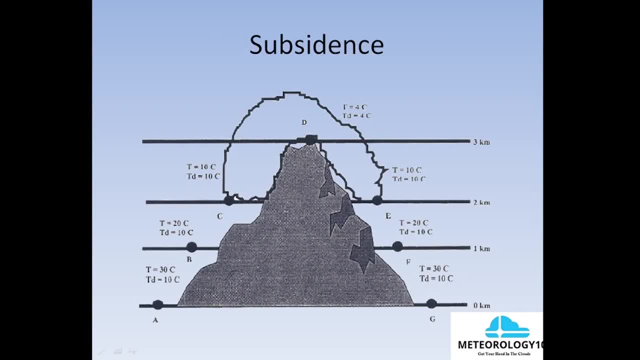 subsidence, but like your lapse rates, your typical lapse rates about six, really about six and a half degrees per thousand feet. it's ten degrees degrees on a dry adiabatic layer level. 10 degrees per thousand kilometers, i'm sorry, a thousand meters, and then six to six and a half degrees after that. so when a partial sinks or subsides, then the 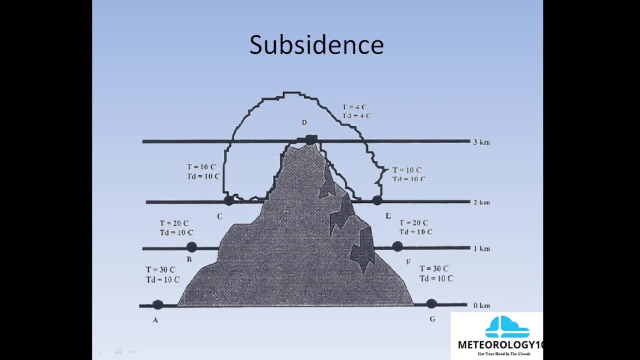 pressure rises and the molecules are packed closer together so that heats that air. so, like the think of the santa ana winds, when they come down the mountain they're actually compressing and warming and you will actually have warmer temperatures on the surface with the wind that comes off the 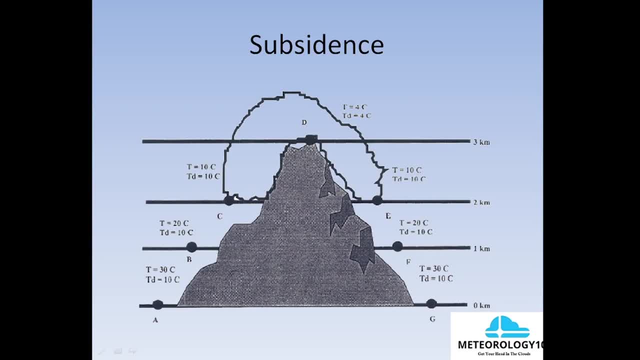 mountains. even though it's a colder air, it will actually compress enough to warm and create that warmer condition on the surface. um, so if an air partial is 30 degrees and risen three kilometers, it will cool 20 degrees and if we force it back to the surface it returns to its original 30 degrees. so that's. 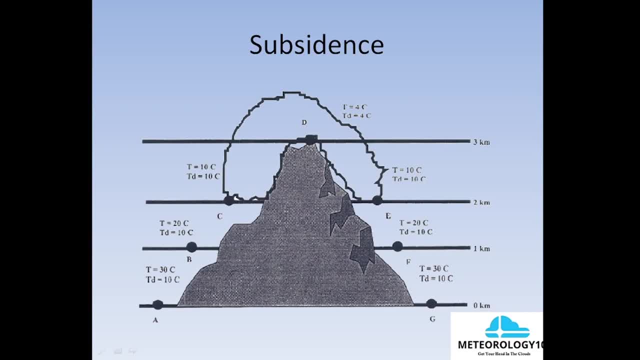 the picture we painted on with this uh lift is what? basically? where that temperature starts is pretty much where it's going to end up on the lee side of the mountains. okay, so if condensation occurs at some point, the liquid droplets are present in the parcel, the parcel. 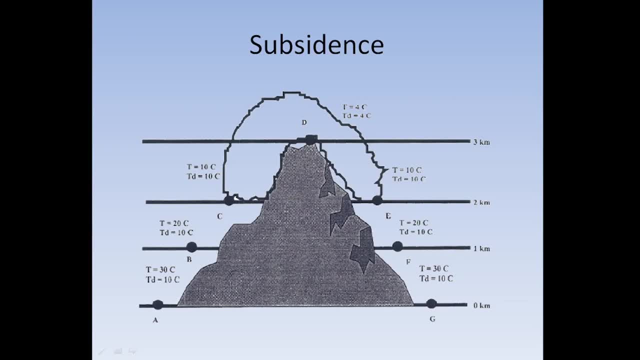 sinks and warms in the droplets, or ice crystals, evaporate back into the parcel, back into the air and no longer it's no longer in a saturated state. so that's when it starts to dry out. so as it descends it, it actually releases the 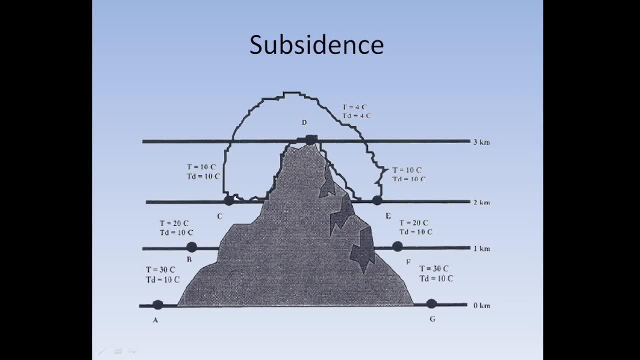 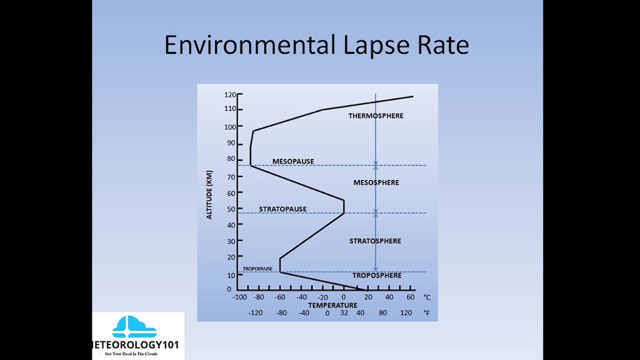 moisture back into the air and then it's no longer saturated. it actually becomes the vapor at that point. so it's a higher energy state, all right. environmental lapse rates. this is a typical layers of the atmosphere. temperature change of the actual atmosphere with height is what the lapse rate is. buoyancy and 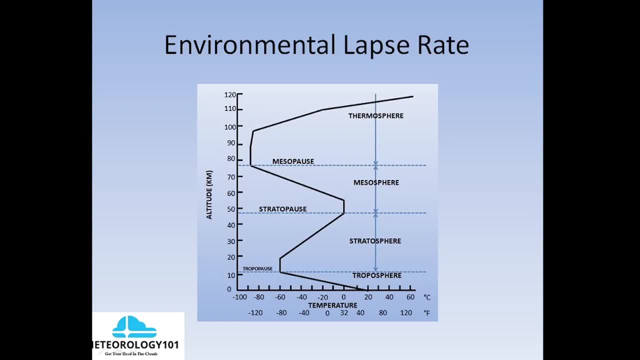 stability are determined when we consider the relationship of dry adiabats, moist adiabats, with the environmental lapse rate. so the environmental lapse rate, like we said, is typically about six, six and a half degrees per 1000 meters. so we live in a troposphere. typically, temperatures decrease with height, so we 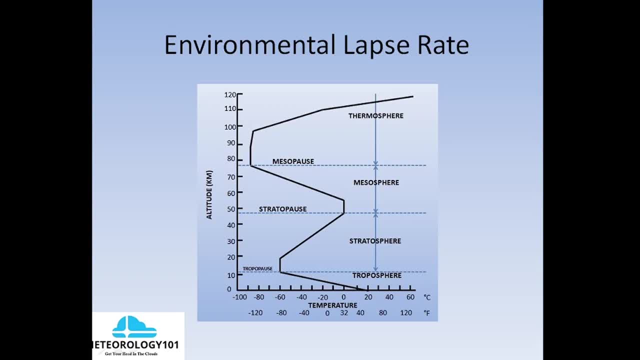 have a positive lapse rate, then once you hit the tropopause, then there's no change in temperature and then there's an increase in temperature. it's a stable atmosphere in the stratosphere. so as far as stability, actually we'll get into stability here in just a few minutes. cold air over warm air is an unstable environment we live in. 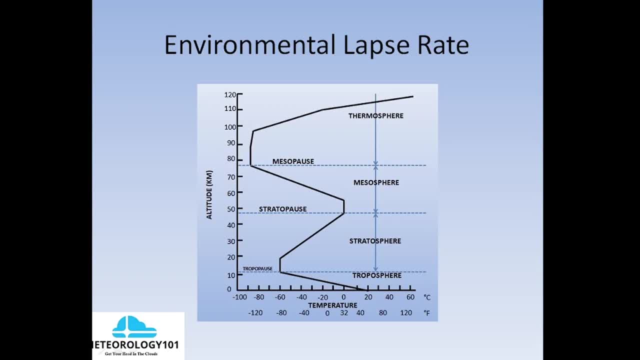 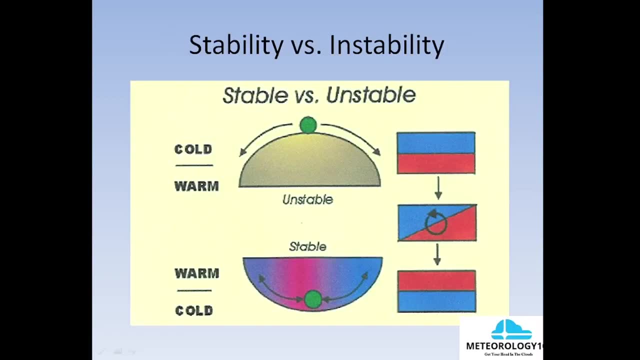 a troposphere. as a we go up in height, it's cold. the cold air continuously wants to sink. so just think of we're in a troposphere, we're in a tropical, we're always in an unstable environment. so there's stability versus instability. cold over warm is unstable because cold air wants to sink if you push that air. 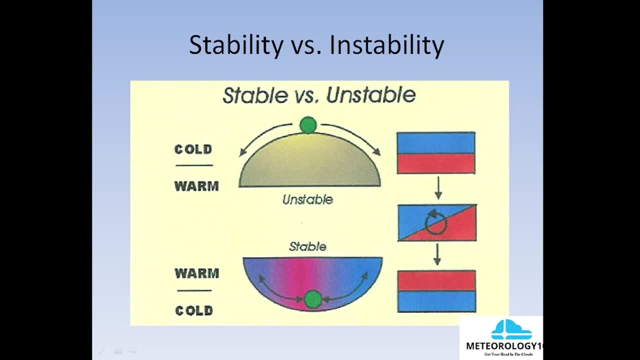 partial cold air partial. it will continue to move in that direction. so we push this ball off the bowl. cold air wants to sink. it's gonna continue to sink. warm air: if you push the warm air up, it's gonna sink. so it's gonna sink in a stable environment. if the warm air is already up and the cold air is down, you push that warm air. 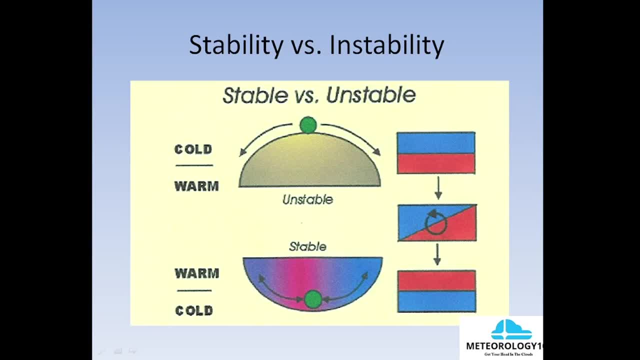 up. it's just it's going to go, stay back, continue to rise, so you're in a stable environment. warm air wants to rise, cold air wants to sink. they're separating, no mixing going on. cold air wants to sink, warm air wants to rise, so you got a lot of mixing going on. so you're in a stable environment. 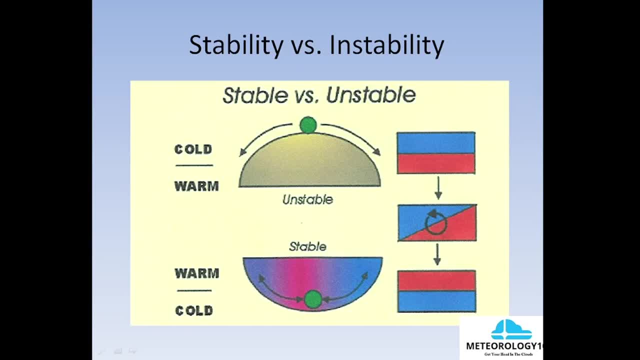 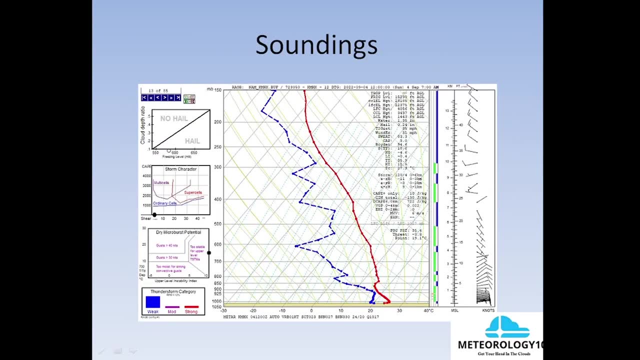 now, if you push an air parcel and it stops and returns to its original position, then you're in a neutral environment, which that does happen to. so all right. so the soundings, um, it's a graph- the properties of the atmosphere, such as temperature, dew point and respect with that. 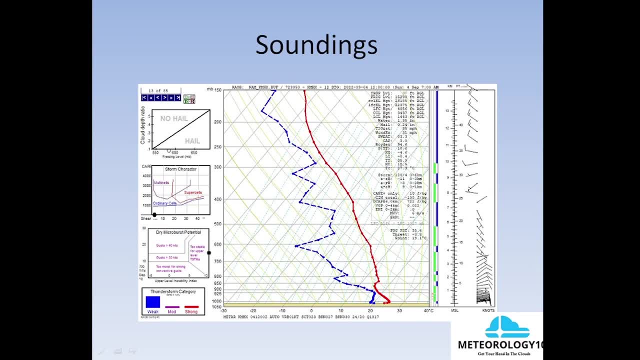 altitude. so um they let the balloon go. radio song sends back all the data. we used to plot these scooties, the scooty log p diagram. we used to plot these by hand. the computer does pretty much everything for you now, so um. that chart was invented in 1947 by meteorologist and physicist nikolai. 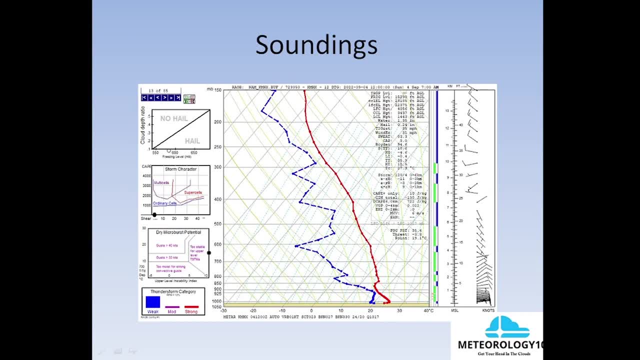 herlifson and was quickly embraced by the united states air force. so when we go to weather school- i was in the military for weather school- we went to the air force weather. they're the ones that did all the weather training and we did learn how to plot. 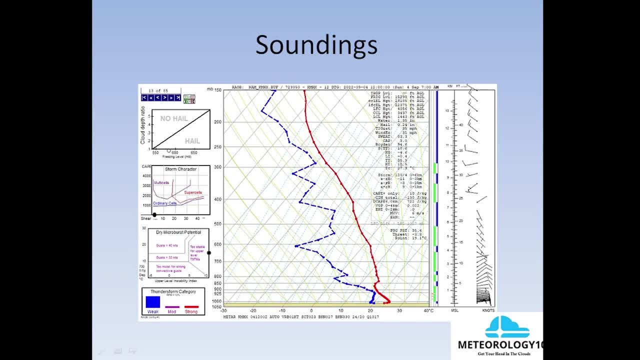 a scooty by hand and then analyze it, all the different readings by hand. but, like i said, now with computers, all the programs out there, we don't have to really do anything by hand. they got rid of all of the dyfax charts that used to print out um from these weather balloons and all that. 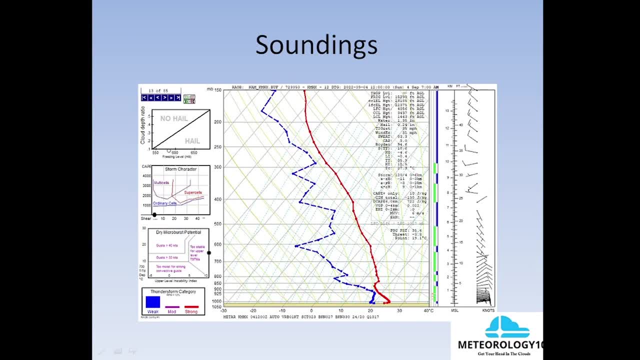 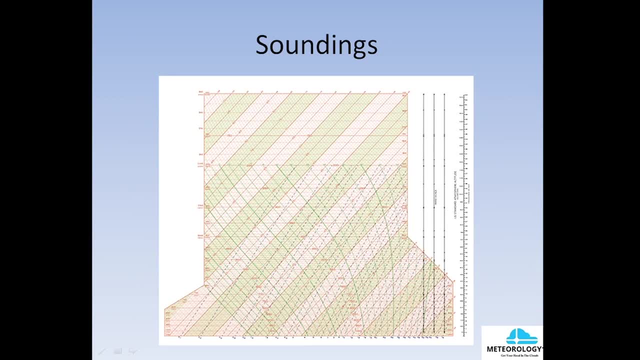 was printed out and we would actually go through and analyze those by hand and uh, that way we got a more accurate forecast for our local area. so sounding or scooty? this is the complete scooty chart. um, we'll go through these lines so you understand what they are. 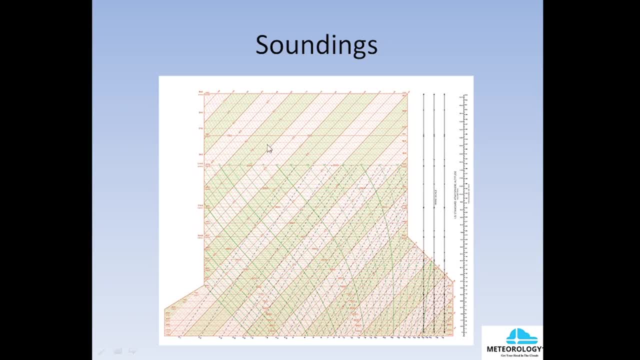 so you got the solid lines going diagonal, solid lines going horizontal, you got the green lines that are kind of skewed and you got the dan green dash lines at an angle also. so, um, if you look at these, this is pretty hard to see, but they're separated by green and kind of a pinkish. 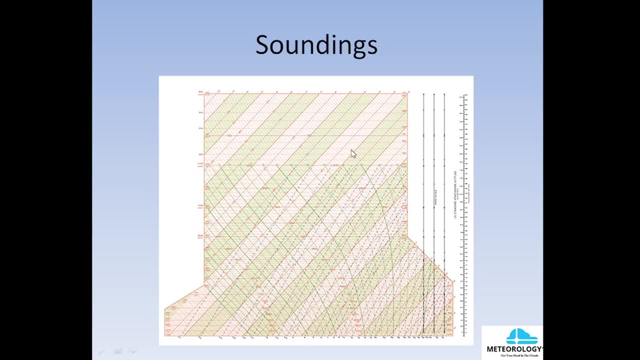 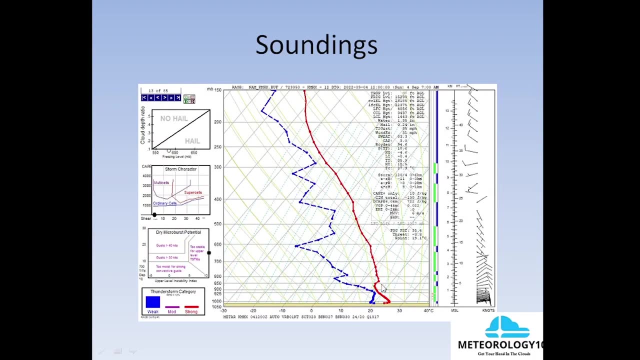 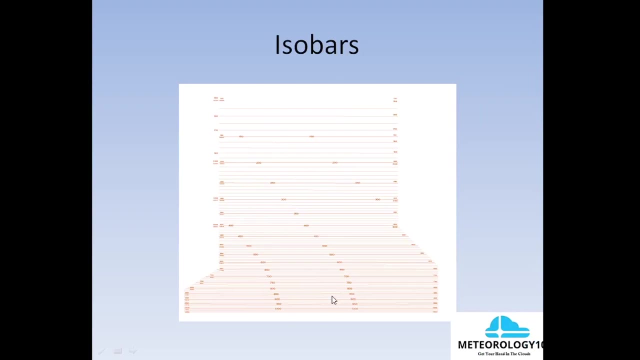 orange um that. those are every 10 degrees, so each section is 10 degrees fahrenheit. so let's go look at these lines. the horizontal lines are solid lines. they're isobars, lines of equal pressure. this is based on a standard atmosphere. so we've got there's a height scale on the left that indicates uh, feet or meters, so you can use either. 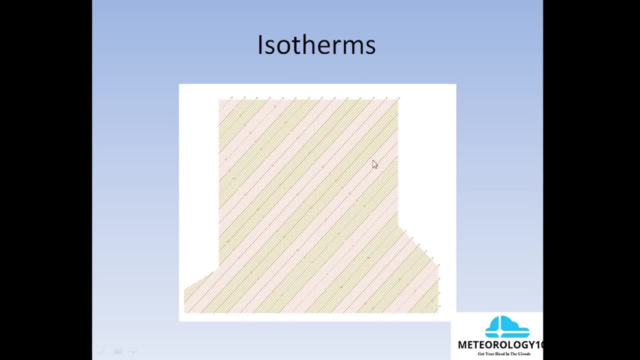 or standard. on this chart the isotherms, the lines of equal temperature for a standard atmosphere, are at an angle and those are the ones separated with color. so those are every, like i said, about every 10 degrees between those different colors, each color section about 10 degrees is 10 degrees. all right, the mixing ratio, the dash lines are: 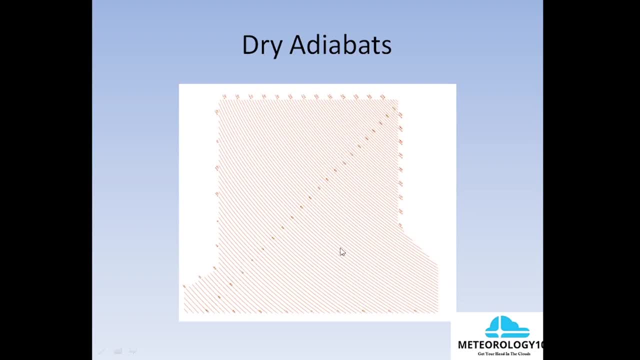 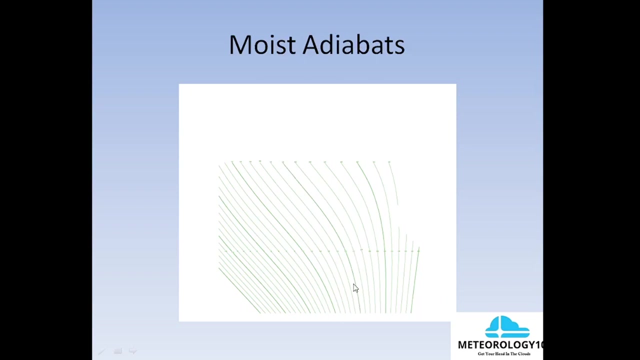 going at an angle. that's the mixing ratio lines, the dry adiabatic lines, those, if you look those skewed up into the atmosphere. they're a solid line going from the bottom right, top left. moist adiabats are skewed line, green line, going pretty much from the bottom of the chart and then it's 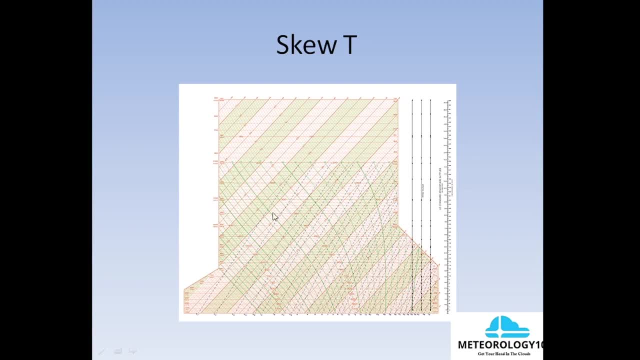 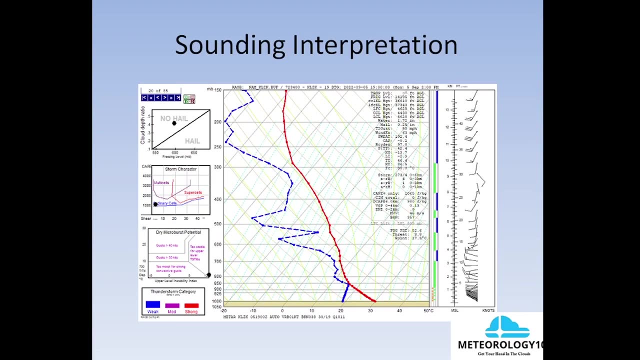 going up to the left of the chart and then that's back to the original completed chart. all right, so what are all these lines doing for us? as we get the data? the data comes in in the code. i don't think i put anything in here on the code. it's um. 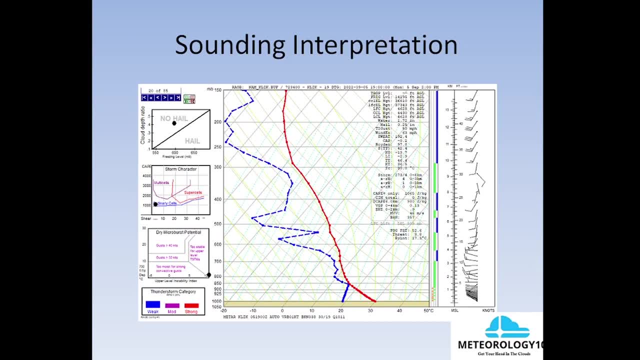 you wouldn't understand if you looked at it without something to break it down. i used to have most of it memorized. we used to plot these things every, every day, twice a day, so you know we could decode that just by looking at it. um, couldn't do it anymore. the uh, but each time 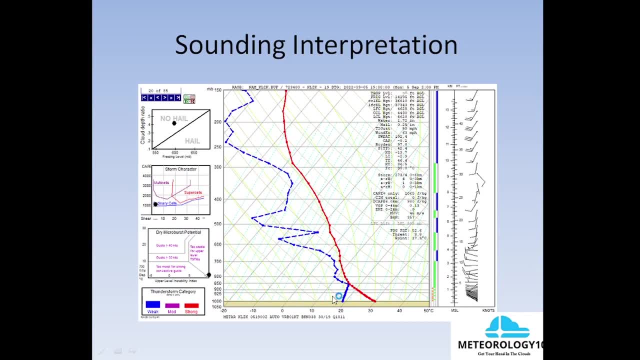 you get a reading. it tells you what level. the balloon sent the reading back at the radio sun center greeting what level it was, what the temperature was, what the dew point was, and then we what the dew points were was and what the uh winds were on that at that level. so you plot temperature. 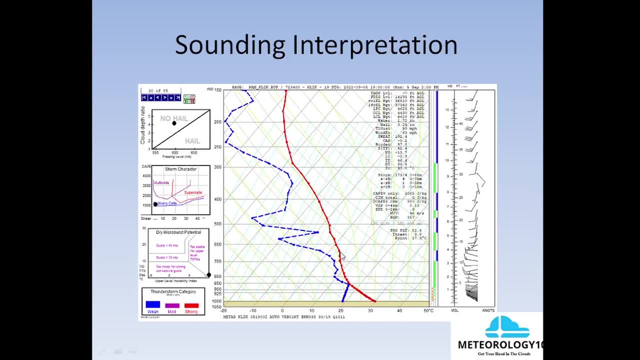 dew point winds on each, each layer, so each one of them dots. is is a height that the balloon has sent data back. so every height you have a plot. the blue is a dew point, red is temperature and then you have your wind bar. now these lines can change. you can go red, blue, red, black, black, black. it really 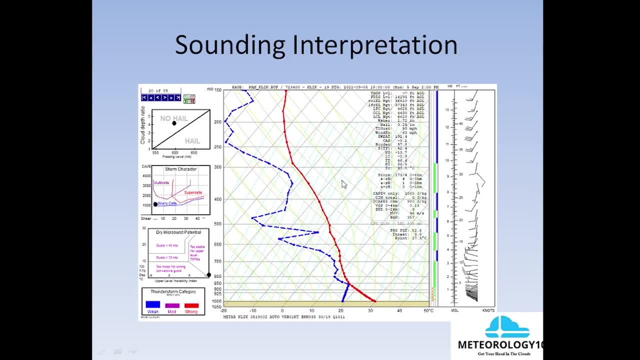 doesn't matter, because the dew point will never cross over to the right of the temperature, will never be higher than temperature they will always be. it will be equal or less. so you always know that the left line is typically a dashed line when that's plotted out, but that line will always be. 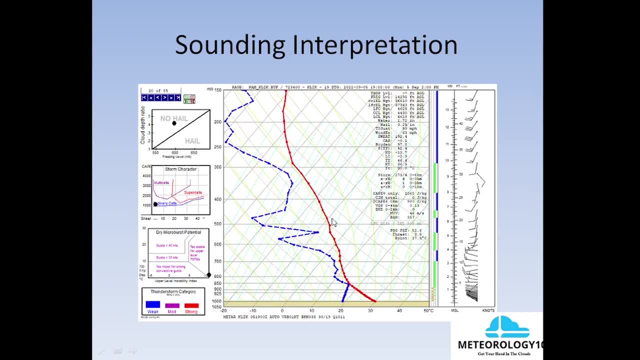 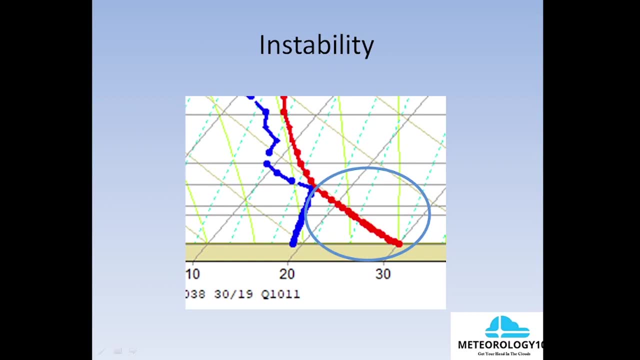 to the left of the temperature instability. now, one big thing on this when we get instability is we were talking about the lapse rates. our typical lapse rate about six, six and a half degrees per per uh thousand meters. so, um, we check how that temperature matches up with the dry adiabats or the moist adiabats, depending on the 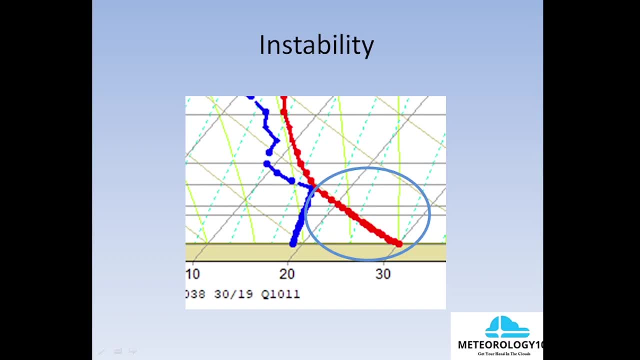 the environment. is it moist out? what's the uh? are we saturated uh? typically, for condensation to occur or saturation to occur, we're going to be typically within a five degree difference between the temperature and the dew point. so if there's a five degree difference or less between the temperature and the dew point, you can say there's significant moisture at that. 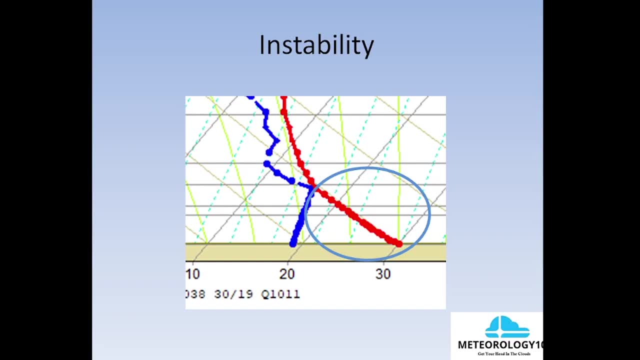 layer at that level, so there's most likely clouds present. we will pull up one of these charts on a computer program i got and we'll see. we'll show you um cloud heights and stuff like that, a couple of different readings and what we get out of it. so um 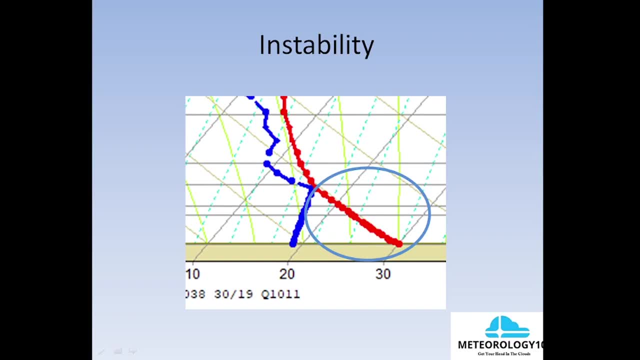 if the temperature line leans forward to the left with height and indicates the layers cools rapidly with height. so you're getting, you're cooling rapidly with height. that is a unstable environment. um, because in our atmosphere we always cool with height. but once you get past that six and a half, 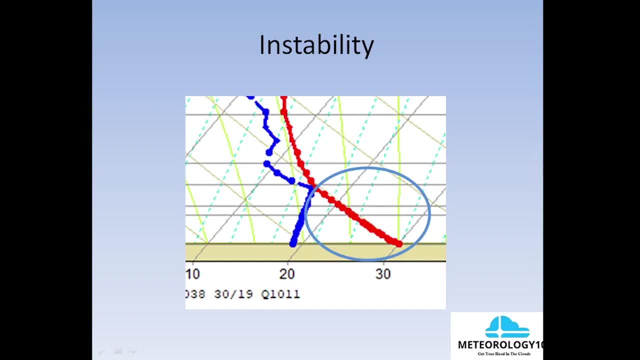 degrees, you start going to seven, eight, nine, you know, ten on the lapse rate, ten degrees per thousand meters on the lapse rate, then you're, you know you're getting into a pretty uh unstable environment. so if the line exceeds both the temperature lines, if it crosses temperature lines or the dry 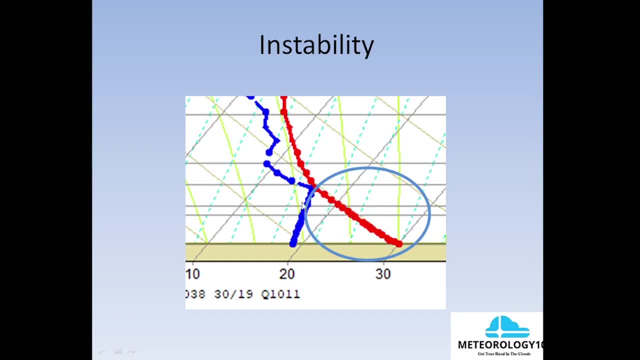 adiabats and the moist adiabats, then you can pretty much say you have an absolutely unstable environment. if it's that steep, like this one, where it's crossing both of these lines, then you are. this is a pretty uh, this is an absolute. it's considered an absolute unstable environment if it falls between the two. 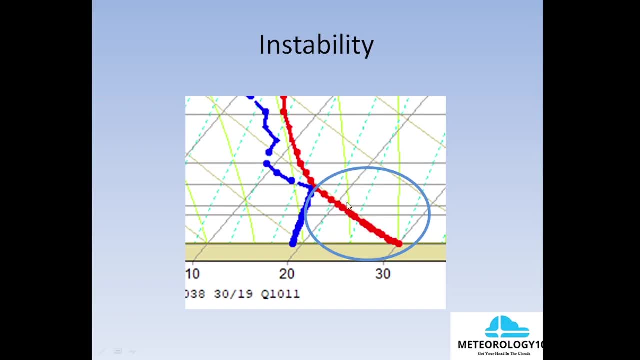 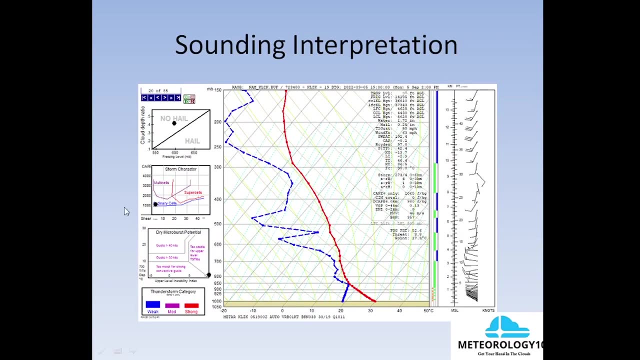 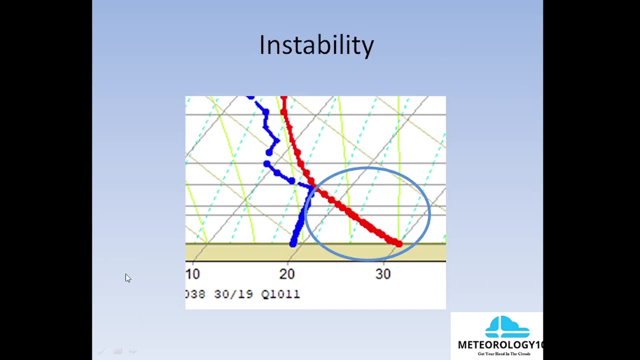 then it's conditionally unstable. so if this was slightly, a little bit steeper, let me see if i have one on the next one, then that's um, that's an inversion, let me go back. so if it's between the two, then it is conditionally unstable, and if it leans to the right of the adiabats, the layer is. 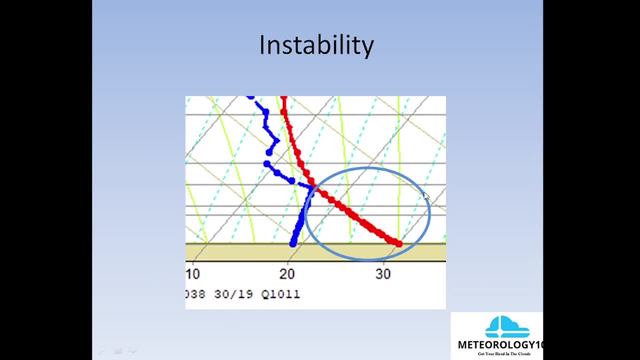 stable. so if the temperature increases with height, we know we're in a stable layer. if we're going almost straight up, then we know we're in a- uh, conditionally unstable layer. and if we're sloping to the left pretty sharp, then we are in a unstable layer. 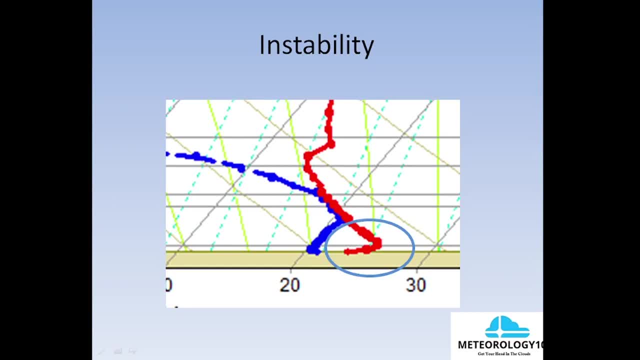 okay, so temperature leans to the right. um, this is a stable error, so i did have it on here. so temperature increases by height. this is an inversion, so it is a negative lapse rate. the temperature increases the height, so you know you're in an absolute stable environment. 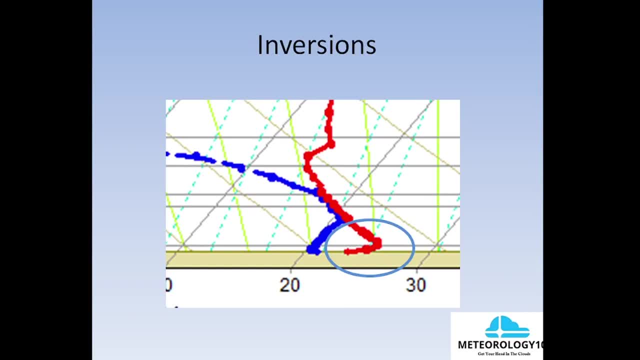 same picture: inversions. that's where the temperature is the same. we're increasing them with height. so if the temperature actually rode with the temperature lines which are right here, these solid lines, if that temperature rode parallel with that kind of gray looking line, or to the right further, then 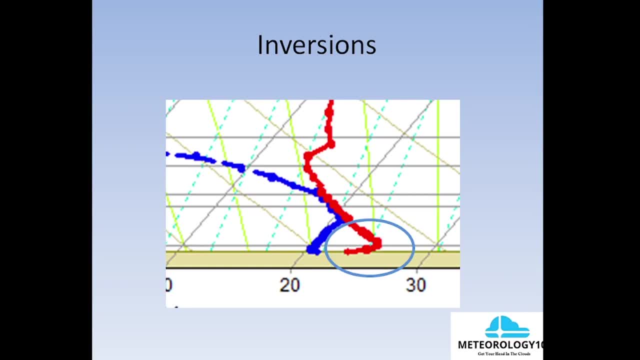 you're in a highly. you're in a stable environment. so the warm air- warm air is above the cool, the cold air, so the cold air is on the surface. you're increasing the height. you have cold to warm over cold. so you're in a stable environment. 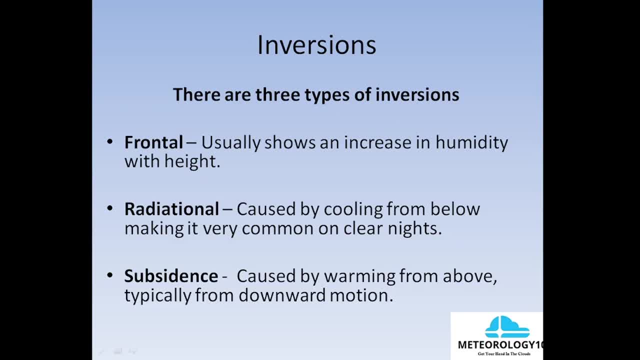 okay, the three types of versions: a frontal inversion, radiational inversion and subsidence inversion. so the frontal inversion usually shows an increase in humidity with height. radiational inversion is caused by the cooling from below, making it very common on clear nights, and then substance aversion is caused by the warming from above, typically from downward. 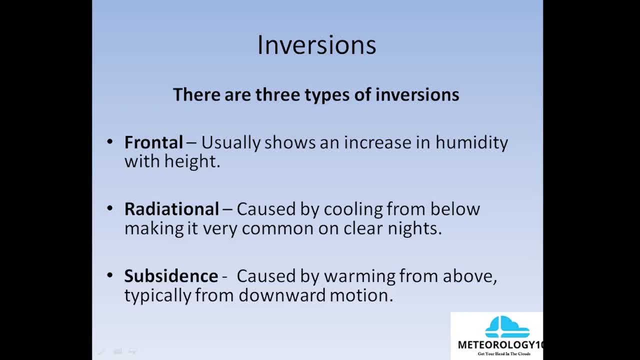 motion. so, like i said, when the winds, sand and winds come off the mountain, they fall, they compress and warm. so as you get that warming you get an increase in temperature and with height the radiational cooling- from cooling from below- you have a warm layer- moves over a cold ground. 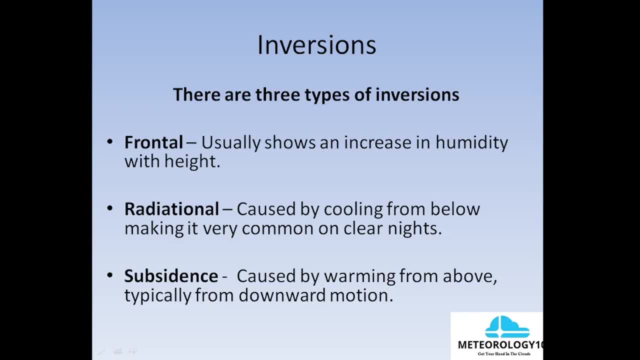 and then it's cooled from below so the temperature on the surface drops. so that gives you a warmer temperature in the upper atmosphere, not real high. we're only talking a few hundred feet or maybe a thousand feet or two thousand feet, but you have an increase in temperature with height. so 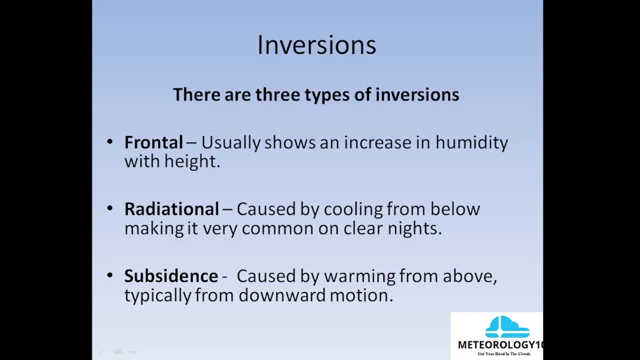 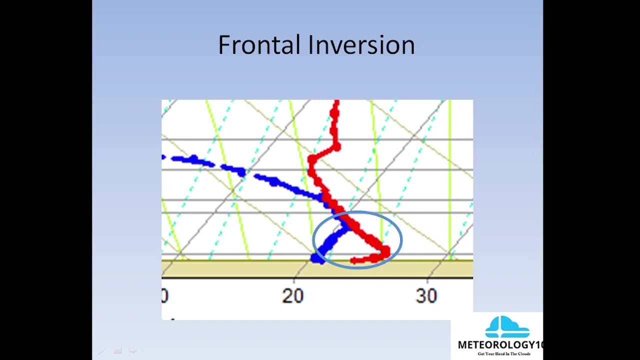 that gives you that stable environment. that's mostly what causes the fog. you get subsidence causing the fog or radiation cooling causing that fog, and then fog is a stratiform cloud on the surface. so it is a stable environment. all right, a frontal inversion. you'll see the um temperature and dew point lines converge with. 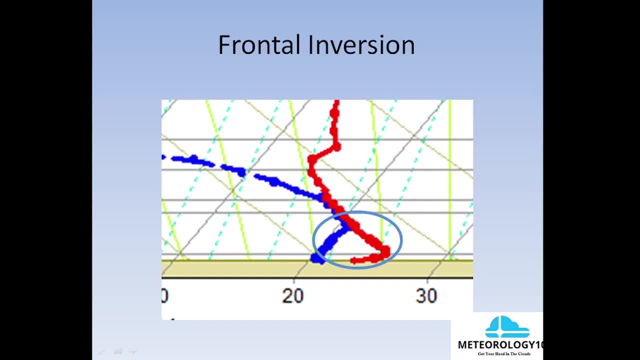 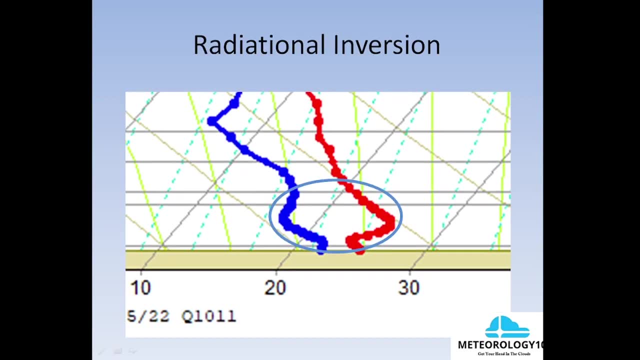 height. that's where both those converge with height. that is the indication of a frontal frontal passage and causing that inversion. radiational inversion is caused by cooling from below, making a very common on clear nights, like we said before, and a decrease in humidity in the inversion layer, and occurs only on the surface. so 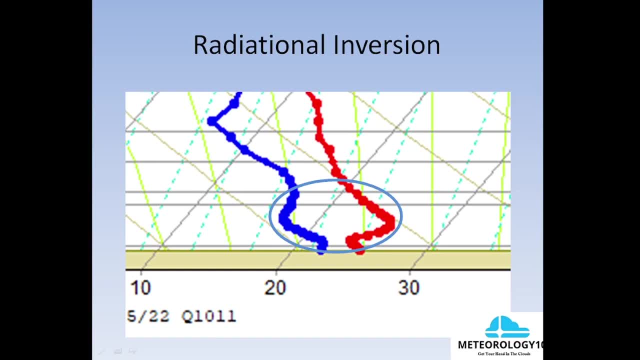 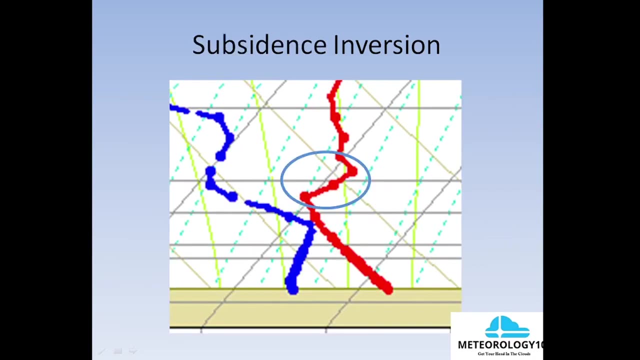 you'll see that warm air moving over a cold surface cooling from below the surface, temperature drops and you'll have that increase in in temperature with height. so that's a little bit of information for you to take a look at. then the subsidence inversion, the way to tell the difference. it pretty much. 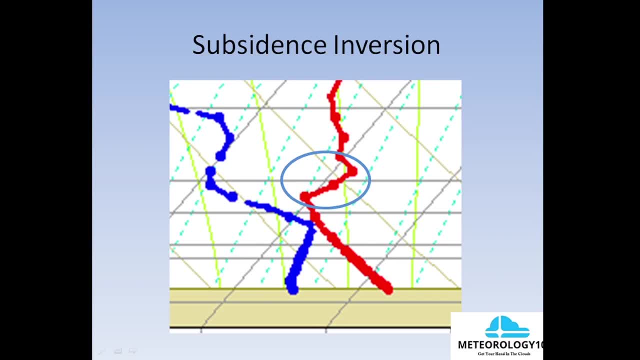 it's almost apparent. this appearance is identical to a radiational inversion on a screw t, but more likely to exist aloft than on the surface. you'll see that in the upper levels, you won't see that on the surface. so we're decreasing with temperature height. then we 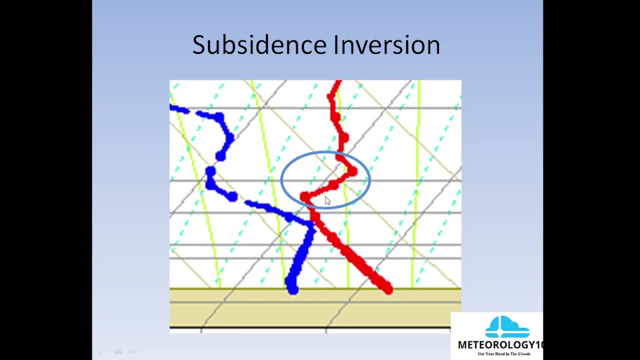 start to increase with temperature. that's a stable layer in the upper atmosphere. you could have rain everything down here, um, with all this moisture, but this is pretty much going to cap that atmosphere. so in a situation like this you can get radio signals a lot further because you have that. 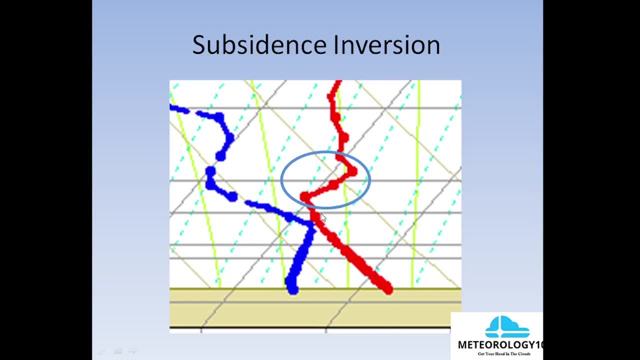 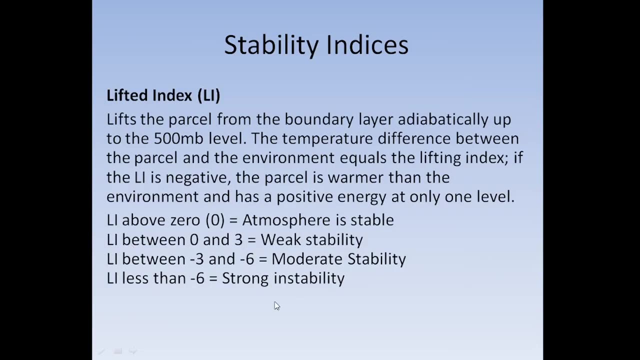 capping going on and radio signals will bounce off of that and then turn to the surface. bounce off the surface and you have a continuous wave going and it'll travel out to a further distance. same thing with noise. all right. so some stability indices that we get from this thing is a lifted. 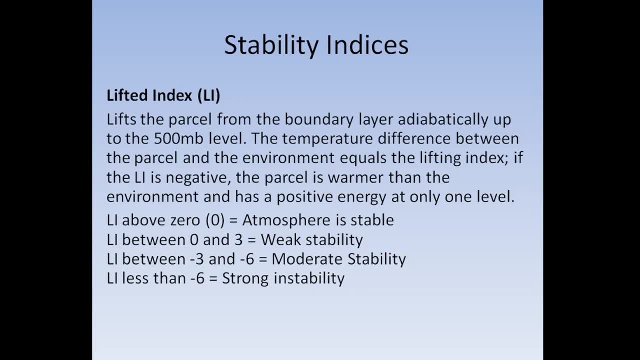 index, um, based on these uh values, what? how stable we are in the atmosphere. so if you want to screenshot this or something- uh, i'm really not going to read all that- we're going to go. uh, look at the values here. so, in a lifted index above zero, the atmosphere is stable and a lifted index 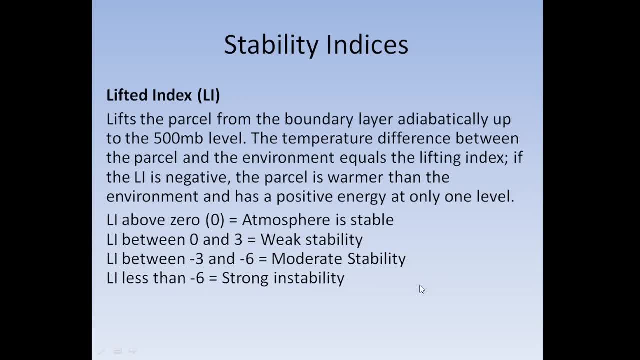 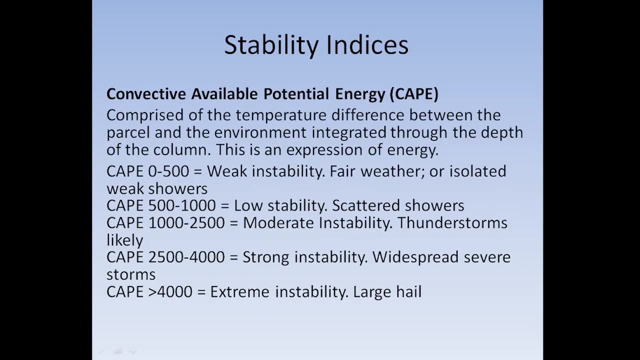 less than negative. six is strongly unstable. it's strong instability. so um, looking at these indexes is one thing. it's one tool to use on this chart to determine the stability in the atmosphere. all right, the uh convective, available potential energy- everybody's heard of this one, the cape. 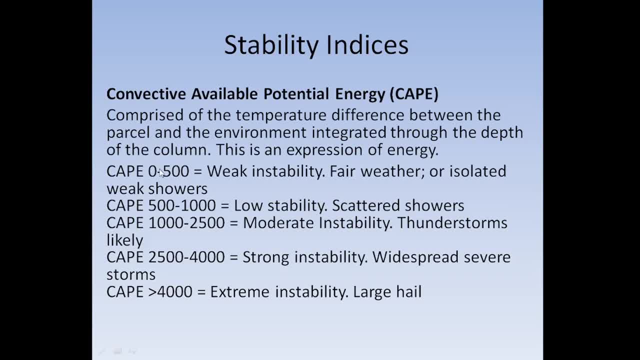 um. so your cape values: zero to 500 is weakened stability. 500 to a thousand low, low stability and then a thousand twenty five hundred moderate. uh instability thunderstorms are likely. 25 to 4 000 strong instability, widespread severe storms and greater than 4 000 extremely unstable to get. 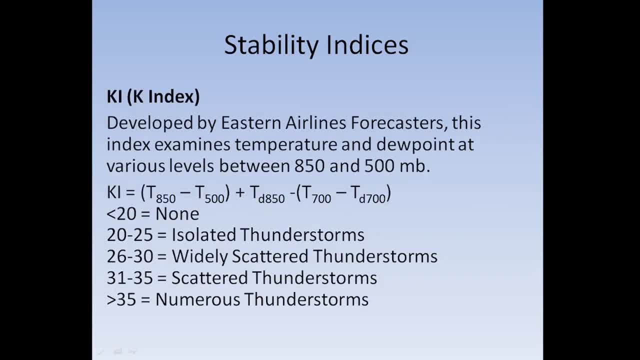 large hail out of that. the ki uh, the k index, um. if you take the upper layers, like the temperature at the 850, minus temperature at the 500 um, plus temperature, dew point temperature at the 850 and minus the temperature to 700, the dew point temperature of the 700, then you end up with this value that gives. 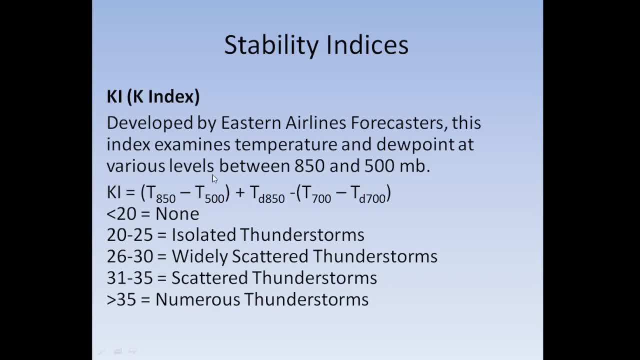 you what you're gonna. let's say you're going to, let's say you get a little bit of a happy mood with that. then you go to the temperature chart and basically what you're gonna end up with these temperatures and the upper layers like that is: do you have a cold over warm situation or? 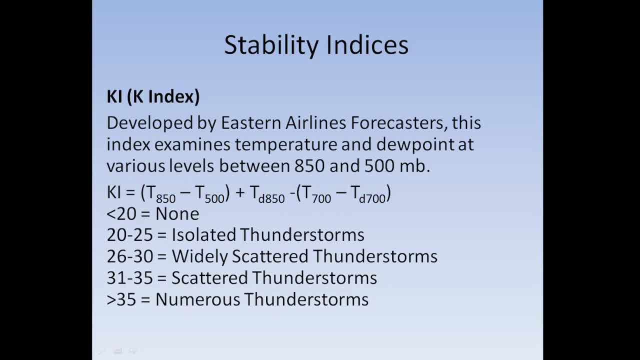 a warm over cold situation. so if your value ends up being less than less than 20, there's no threat of instability, no threat of thunder. storms: 20- 25 isolated, 26 to 30. widely scattered thunderstorms: 31 to 35. so, like i said, there's no reason to calculate this. all these computer systems do it now. 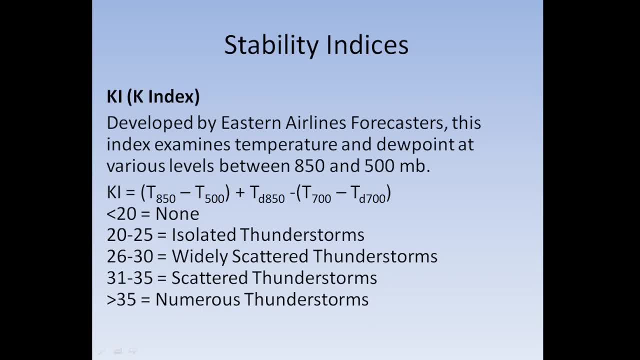 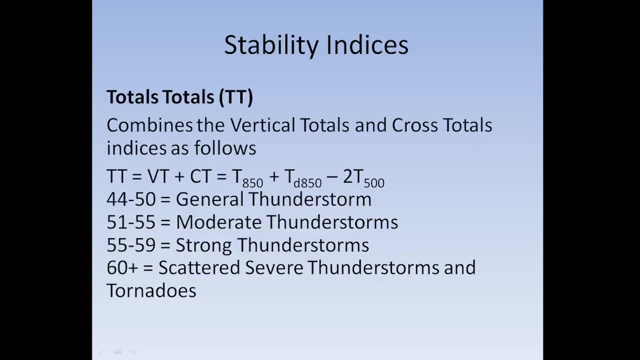 we used to have to have to do it, now we don't. so figure out these indexes pretty much like I said. the computer program will tell you everything you need to know: total totals. another instability tool to use on this chart and low-level jet- definitely I need need. 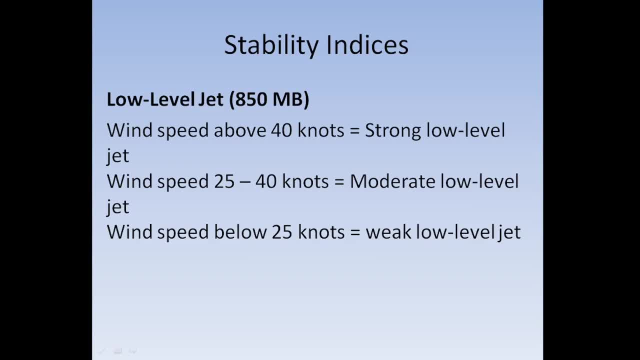 to know if you have a low-level jet. that's going to tell you basically: do you have a strong low-level jet, moderate a week? because that's going to give you an idea of what your wind shear is on lower levels if you got lower level jet. 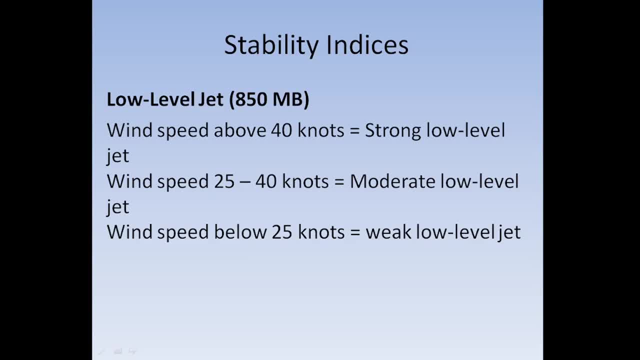 or you know, 40 knots or greater, at the 850 millibars you have a strong low level jet. so once you hit that level, then you have a surface low or a thunderstorm and you have that low-level jet feeding that thunderstorm or pulling. 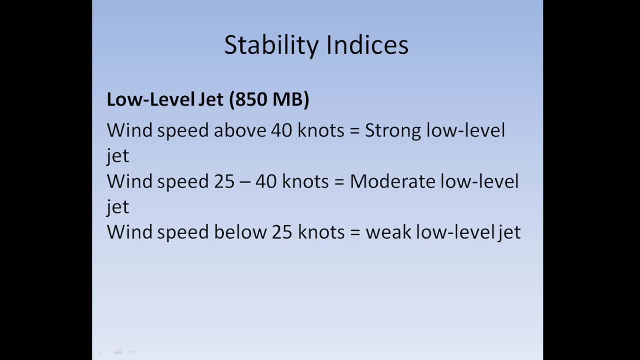 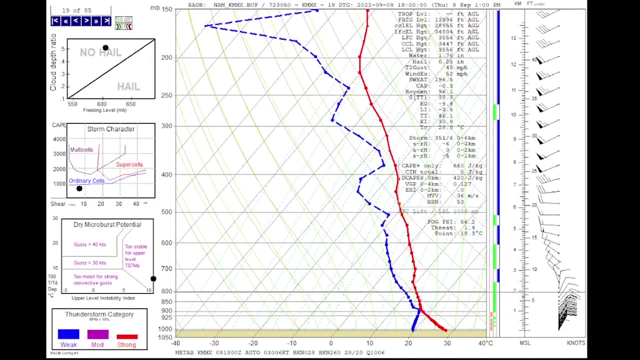 the mass out of that thunderstorm, then you can have a very strong updraft and you can have severe weather tornadoes, because you have a low-level jet present. so good to know if you have 40 knots at 850 millibars right right around 5,000 feet, all right, let's get. 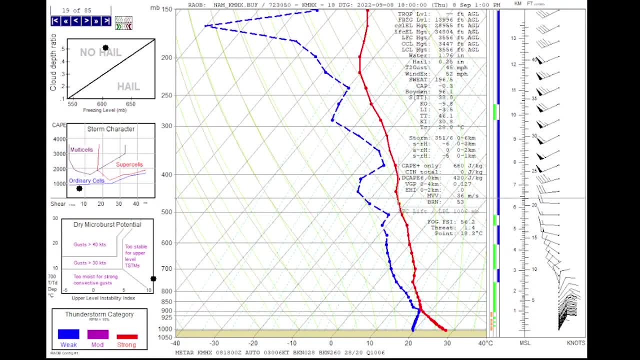 into the soundings. so this is your typical scooty chart. this is the program. it's a ray of software, a little bit pricey, but you can pull up scooties anywhere across the United States and this software will analyze them and download the, the model data, so you can do forecasts- scooties also- and then try. 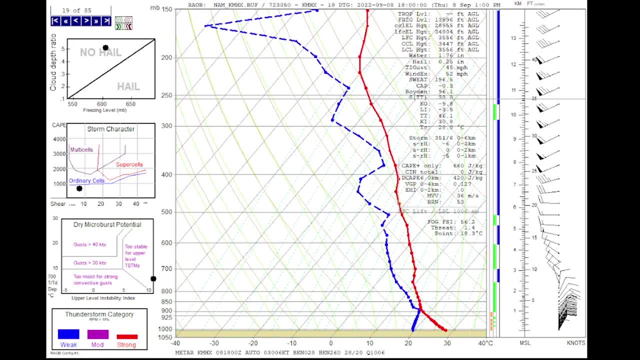 to pinpoint where your thunderstorms or super cells are going to hit, based on each station. so take some time to do all that. but as far as plotting these things, a computer plots everything for you, analyzes everything for you. we got a whole list of numbers on the right-hand side with our all of our analysis and 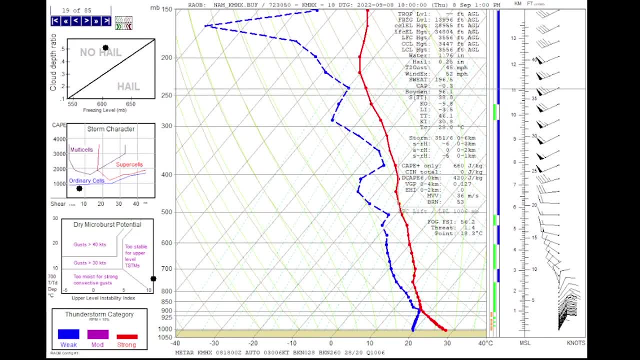 all of the settings here, the indexes for possible severe weather, possible thunderstorms. we're going to touch base on some of these, but not all of them. pretty much we get most of our answers over here and on the left hand side for analysis. give a dry microburst. 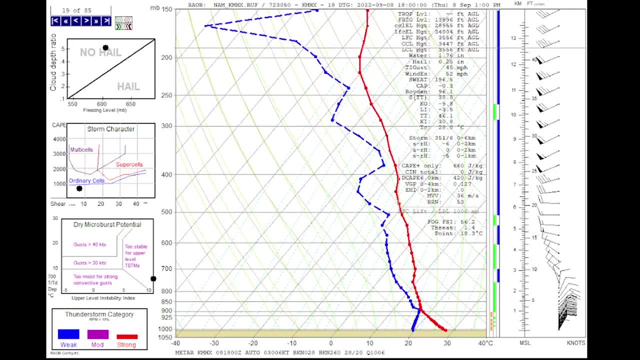 possible storm character and then if you got hail wherever that black dot is, that's what you're you should expect at this time on this scooty. so no hail. this is a sounding for KMHX. it's for a New Bern, North Carolina. it's close to the. 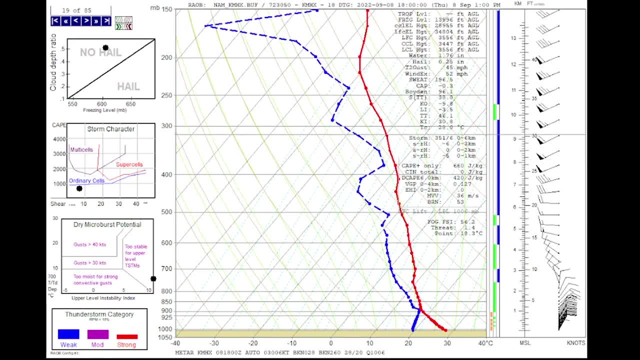 Outer Banks. so storm character where that black dot is. ordinary cells of any thunderstorms popped up in this area right now would just be ordinary thunderstorm cells, nothing significant. so you can go multi cells and then super cells and then there is one area where there's crossover. so if that black dot 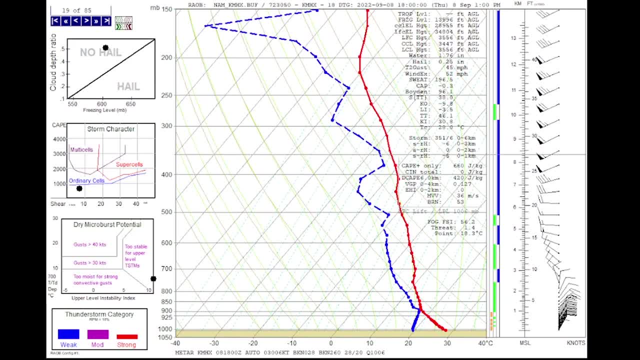 got up into this area. between those, then you'll have- you can have- multiple supercells. um chances that happen pretty slim. but we'll cover some of these indexes, some of the analysis on this. so, um the Trope level, it's off the chart, doesn't even. 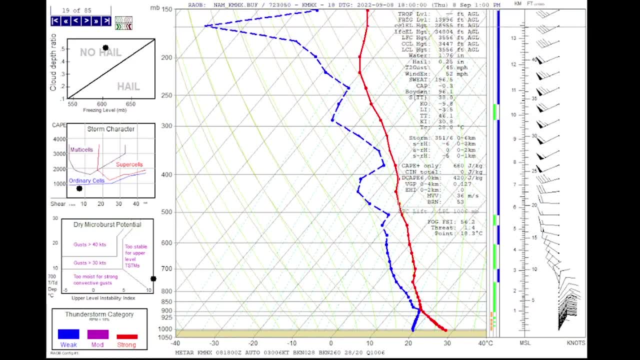 show what the height, the triple troposphere, the top of the troposphere is, the tropic halls, freezing level 13,996 feet. now we can do hit, analyze and then we can work quite complex meters point wise and we canCRB Nina be months. uh, we got quite a bit of different things we could put on here, but we can do. 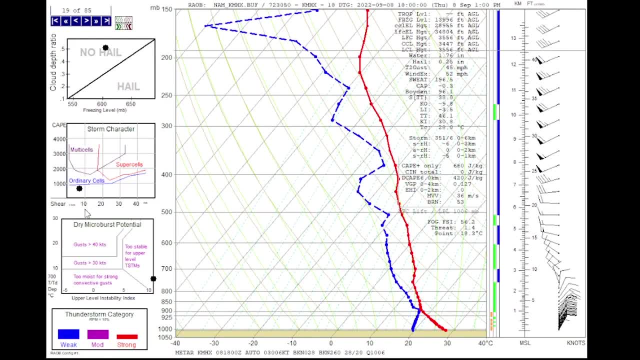 pretty sure freezing level is on here, mixing height, freezing line right there. so now we know our freezing line is right around exactly what that says: 13,996 feet. so you can just get a visual on that, so you can see where your moisture is, how far your moisture goes up, and then you know. 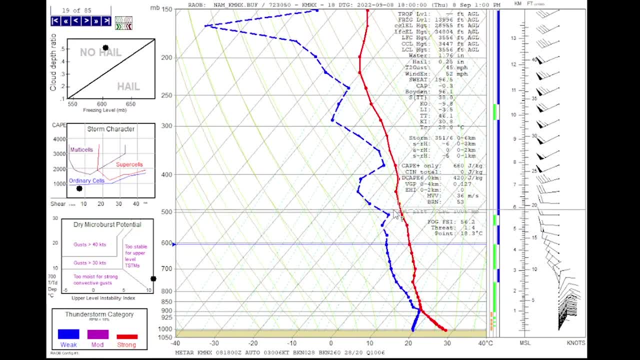 say: okay, if the thunderstorm pops up in this, we're probably going to have hail, because we have enough moisture in those mid-levels to produce that. now hail would be a quarter inch based on this scooty water atmospheric. how much water is in this atmosphere is 1.76 inches if it. 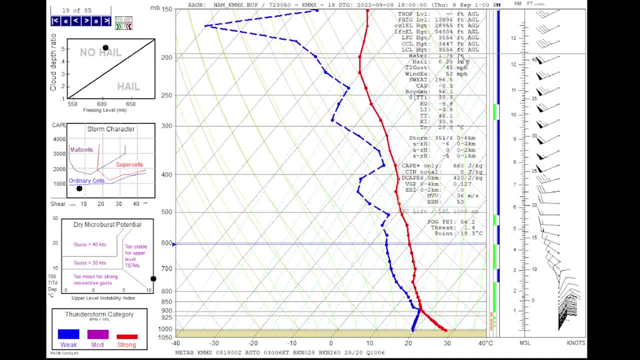 were to rain, how much rain could you get out of it? lifting condensation level: if we lift, lifted a parcel by a terrain or front, a front, anything that gives us, you know, mechanical lift, then what our lifting condensation level is and that's just what level the clouds are going to form. if this was that air parcel was pushed, mechanically pushed, 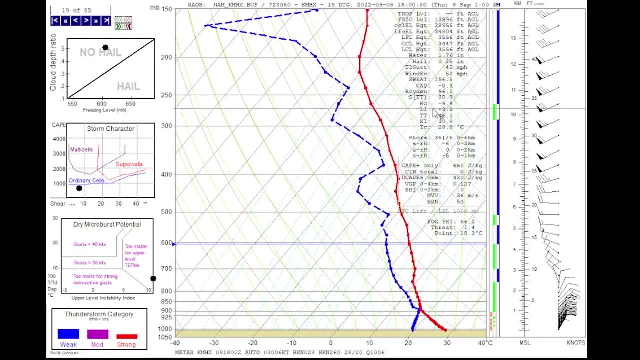 up into the atmosphere. the ccl is the convective condensation level. so if just by daytime heating, heating from the sun, the ground gets hot air. hot air rises, what level would it have to rise to to create clouds? now, in our analysis we can do. we have clouds in here, so now we can see the different cloud layers that we can have pretty 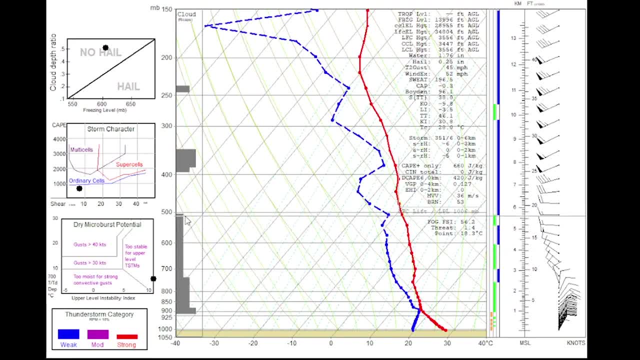 much, all the way up to 500 millibars, which is just over 18 000 feet. that says probably about 18 000 is just below the 500 millibar level. just above 400 millibars is over 23 000 feet. so we have 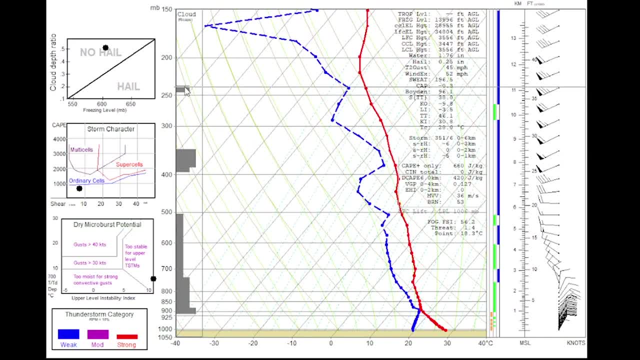 some high clouds and then the 25 000 millibar um 250 millibar level, that's 33, but right at 34 000 feet. so um could have some clouds in that level too. so based on just looking at clouds now we can analyze our 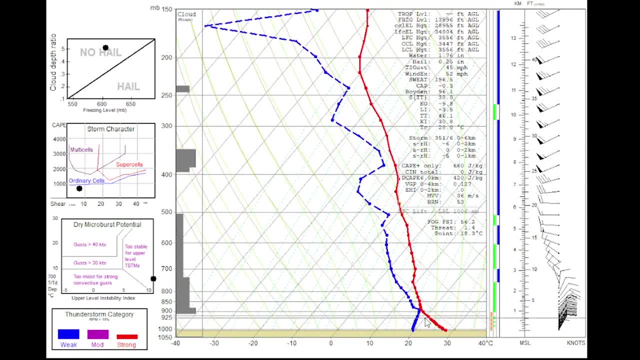 lifting condensation level. basically, you take the surface temperature and follow the dry area back up, and then you take your dew point, surface temperature, your dew point, and follow that moist area back up, and where they hit is where you're going to have your lifting condensation level or your ccl. let's go look at. 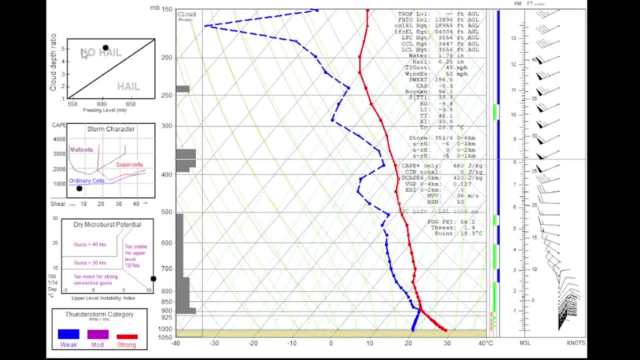 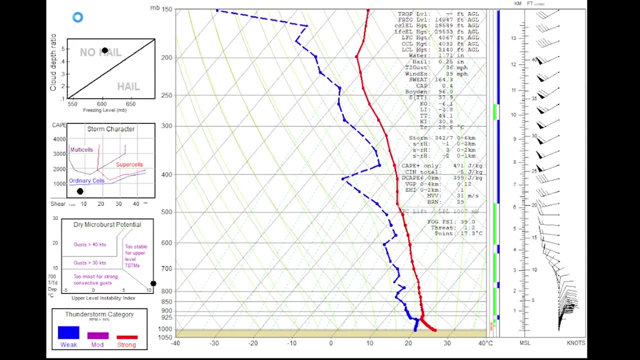 the lifting parcel right there. it's pretty much right. where there's a convergent, there's temperature and dew point. so this isn't a great example, because it's pretty much already giving you the answer there. so, um, i can back these off and open those up a. 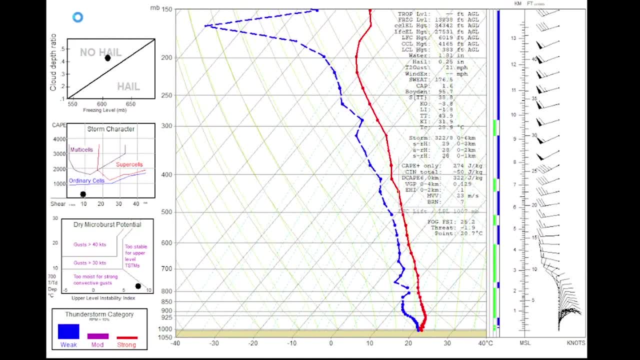 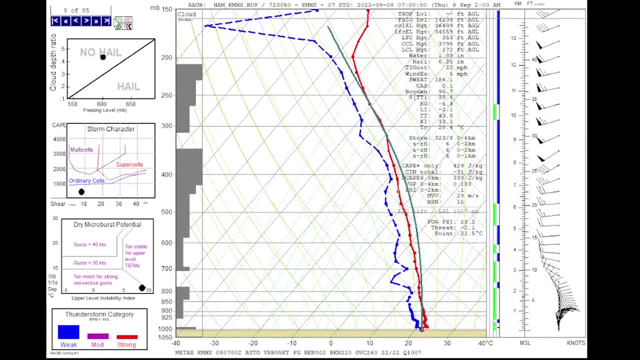 little bit. i was using that one for a uh, more or less for a severe level. uh, look at some severe weather, but not really any severe weather on that chart. just uh, wanted to show you the cape and go through some of those indexes. let's go back forward to this thing so. 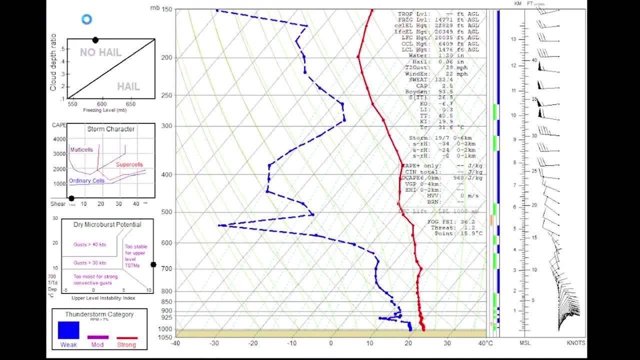 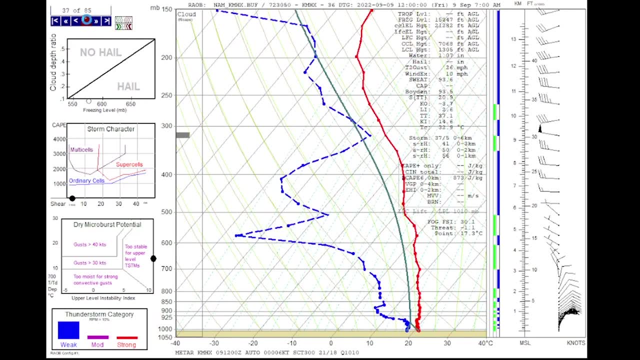 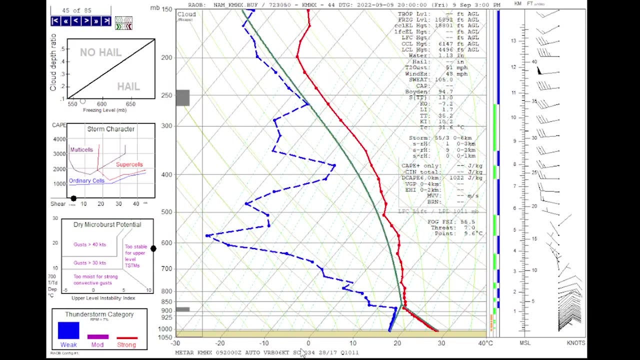 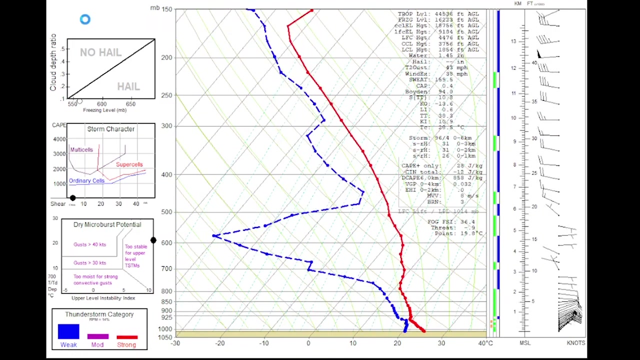 i want to try to get that, um, that lifting condensation level where it's a little bit more visible. it's pretty moist, been pretty moist on the surface. it looks like in north carolina, so, all right, so you can kind of see it there. all right, so that one ain't working out too good. it's, uh, pretty much staying. 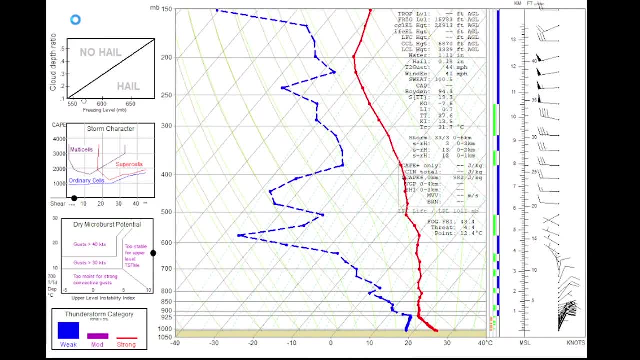 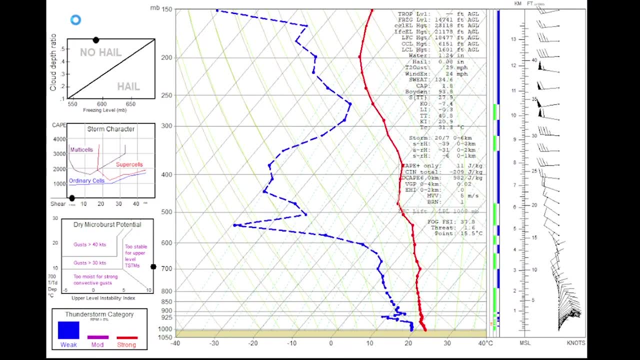 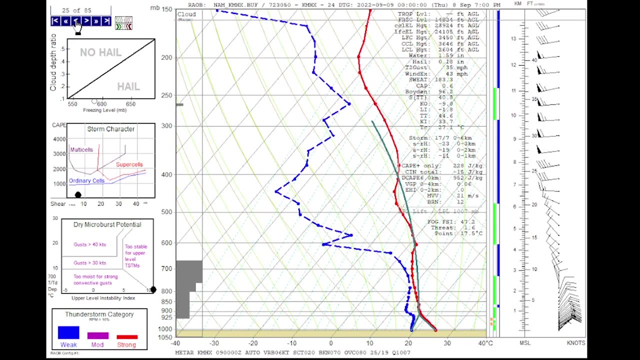 moist, uh close to the surface over north carolina for a little while. let's go to get back to one we want to see. i want to see the cape index. the cape is one that uh most work actually used for severe weather. what's the energy? it's a measure of energy in the atmosphere. 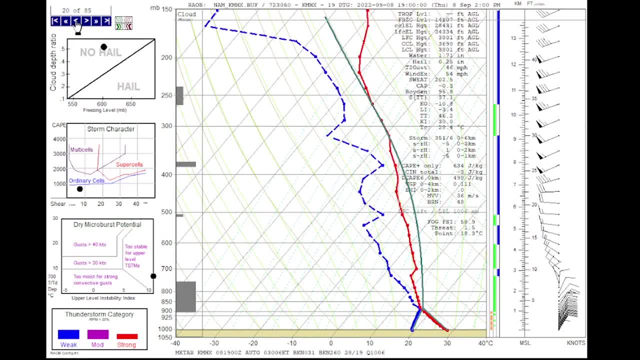 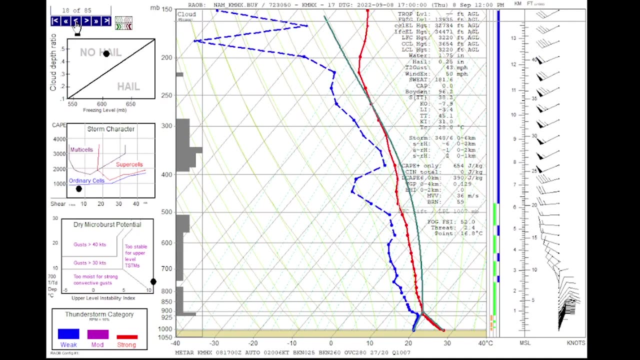 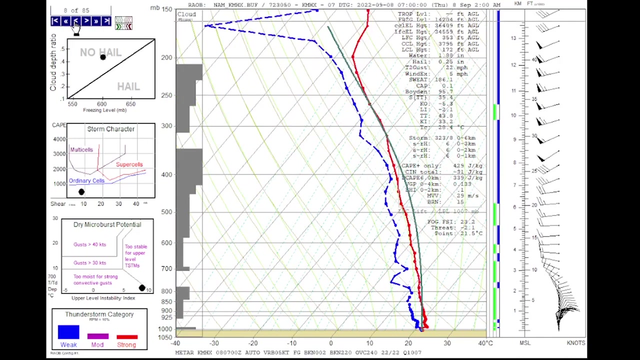 um, we're looking for um a thousand to twenty five hundred joules to be moderate- uh, moderate thunderstorms. twenty five to four thousand to be widespread, severe thunderstorms and then greater than four thousand extreme and large hail producers. so get to a point where we can get see that, basically that lifting condensation level. 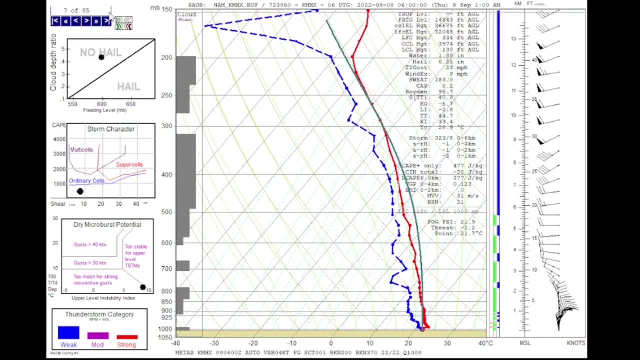 once you start seeing that on the right side of the temperature is pretty much where you're going to have your cape. so we got right there. it colors it in positive cape, negative capes, or energy all down through that, all through those mid layers. um, looking at the uh. 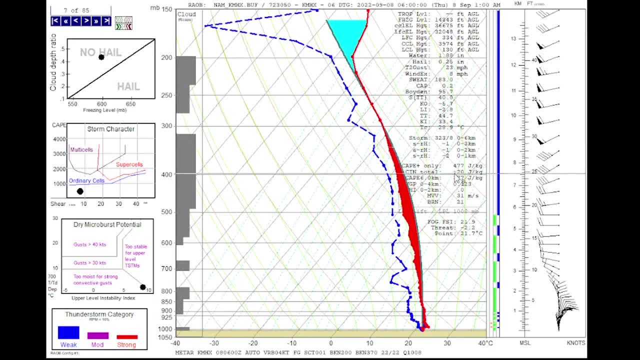 value we got 477 joules, so we're not even close to being uh anywhere for any kind of thunderstorm at severe weather. on this thing all right. when you look at our cloud layers you can see all the moisture, how close these temperature and dew point lines are. 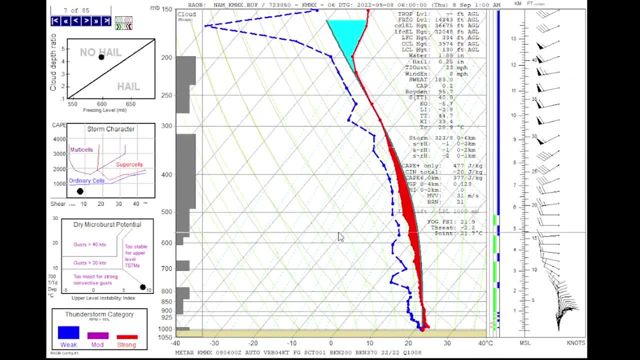 together so you got moisture all the way up into the upper layers. so this actually forecasts out a meter. so you're looking at variable winds at 4 knots with fog, so visibility would have to be dropped less than 5 eighths of a mile to. 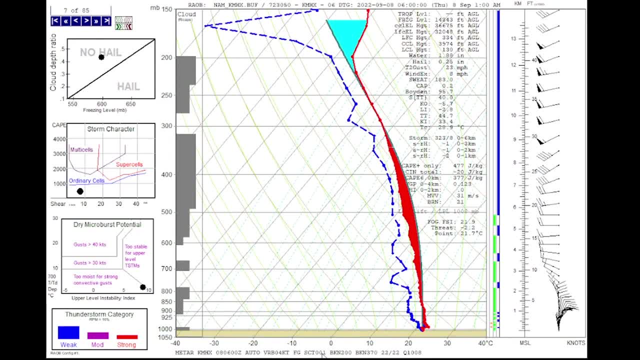 be considered fog, so your visibility is gonna be down, scattered, 100 feet, broken at 20,000, broken at 37,000. now, that's not going to be accurate. I wouldn't think, just because, looking at this layer right here, about 600 millibars are. 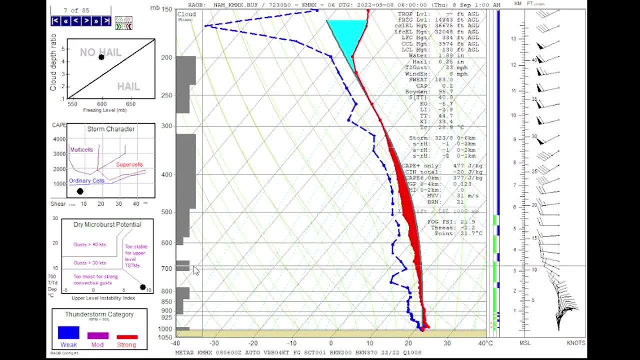 probably about 20,000 feet. 700 millibars are about 9- 10,000 feet, so you should see some clouds in those layers too. so this thing's a broken 20, broken 37, whatever that's like I said, take that with a grain of salt. on the cloud heights now lifted index, the 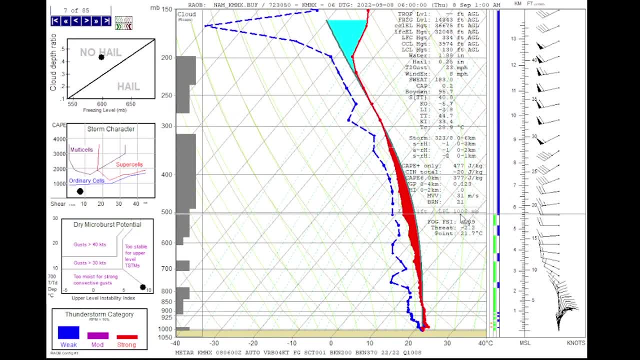 negative 2.8. so we look at their chart and we had lifted index: negative 2.8. you're gonna be a negative. you know. 0 to negative 2 be thunderstorms possible. good trigger mechanism needed so you're gonna have to have something that. 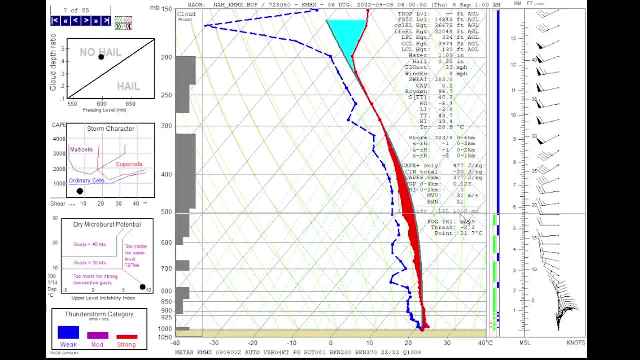 gives you the lift. you need three things for a thunderstorm: moisture, instability and lift. so if you have the moisture and instability, you're gonna have your lifted index. but you need a trigger. you gotta have something that causes that lift. negative, 3, negative 5: unstable thunderstorms probable and less. 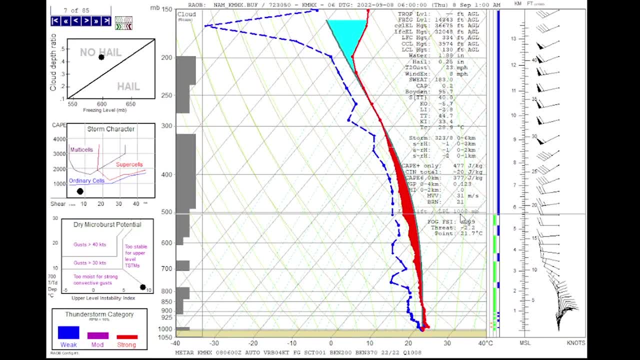 than a negative. 5 is very unstable and as heavy to strong thunderstorm potential. so we're on the weak side of that. but we're gonna have to have some sort of lifting mechanism that will give you the lift to cause that thunderstorm to kick off. so the sweat index: there's a 183. that's another one we 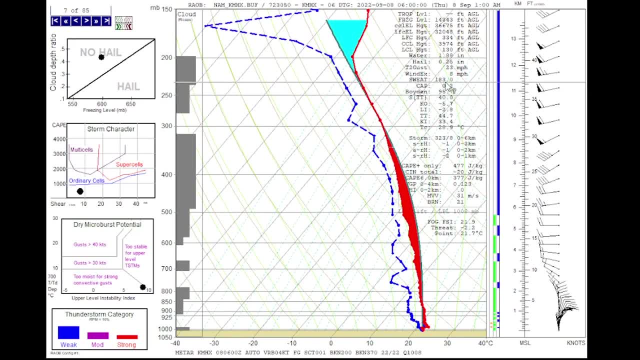 use um zero to 299 severe storms not expected. so if we did get a thunderstorm pop up in this area then we would not expect any anything to be severe. our base level, even our ccl, just from daytime heating- uh, the clouds should be right around 3974 feet, so just around 4 000 feet level of free. 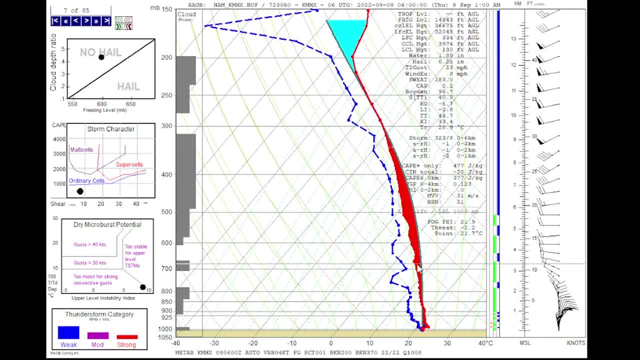 convections at 334 feet. so as soon as that convection, if it did kick off on the surface and all it has to do is hit 334 feet, that's got free convection to continue. nothing's really hindering that. you got a freezing level 14 000 feet. so range option would have to be pushed up that high from. 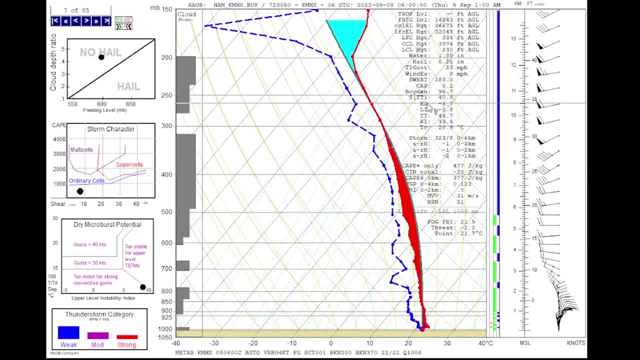 an updraft to get pushed up over 14 000 feet above the freezing level to create any kind of hail. like i said, quarter inch tail would be what we would expect off this sounding, and then the let's see what else we got. total totals 44. uh. 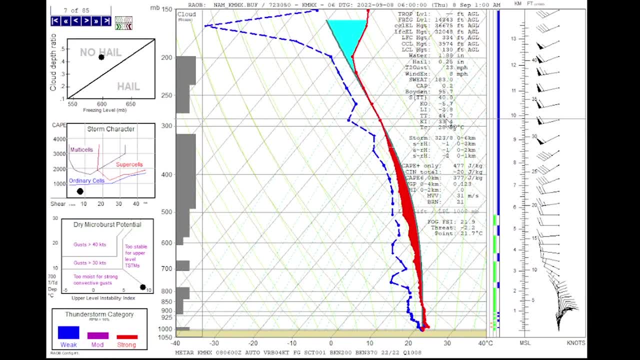 seven, forty, forty, fifty, general thunderstorms. so if a thunderstorm was a kickoff, it'd just be your garden variety thunderstorm, um ki is uh. the k index that one is 33.4, so anywhere from 26 to 30. if 31, 35 scattered thunderstorms. so if thunderstorms 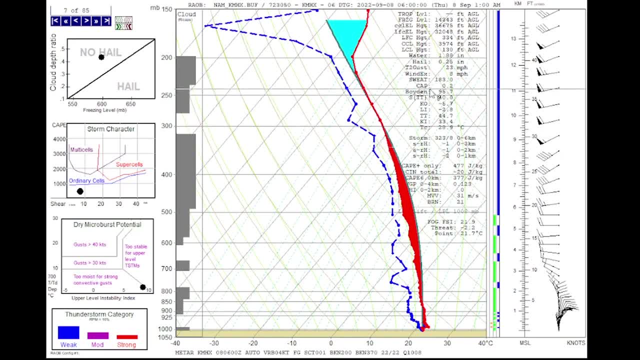 popped up. you could expect them to be scattered, but nothing severe, nothing crazy. so that's why that's what these are all used for, but i take a lot of those with a grain of salt. not all that's going to hit every single time. a lot of other factors we're looking at, so 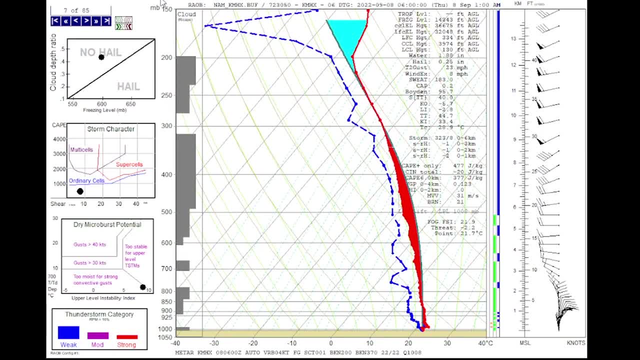 um, let's do an analysis on this thing. let's see what we got, for we can see the cape or cape is. we know we don't have enough energy for severe potential. let's go contrails. where would your contrails be? 20 000 feet or higher, or actually 200 millibars or higher, so you'd that would be up, uh. 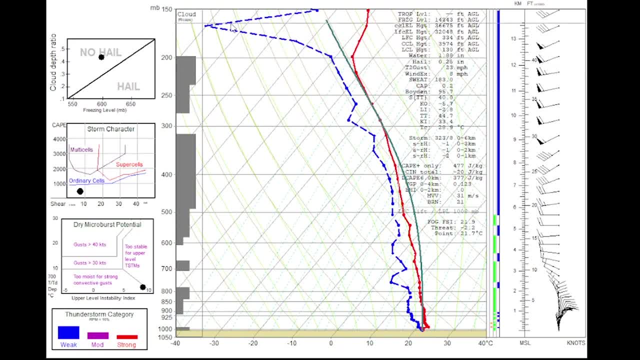 38 000 feet or higher. if if you had a aircraft in that area, they would leave contrails inversions there's um. this looks like an inversion on the surface subsidence inversion of 568 feet above ground level. so this program does tell you what type of inversion you have. 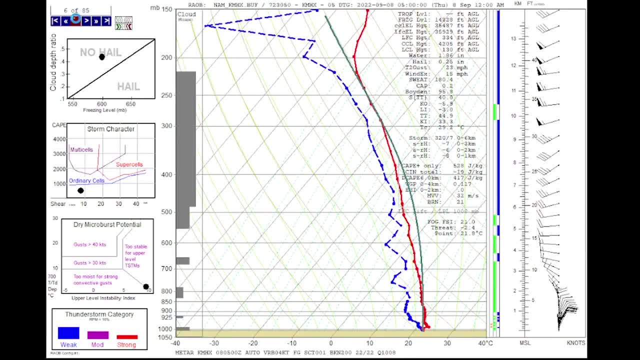 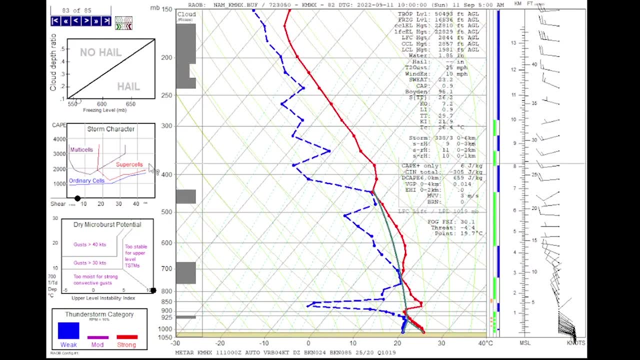 if we back this up and go see if we could pull one where we get to an inversion. right, there's one. now analyze, go to inversion. there we go subsidence inversion, and i can't tell what that is. let me get rid of the clouds. 4395 feet. so with an inversion that strong, uh, definitely a substance inversion being elevated. 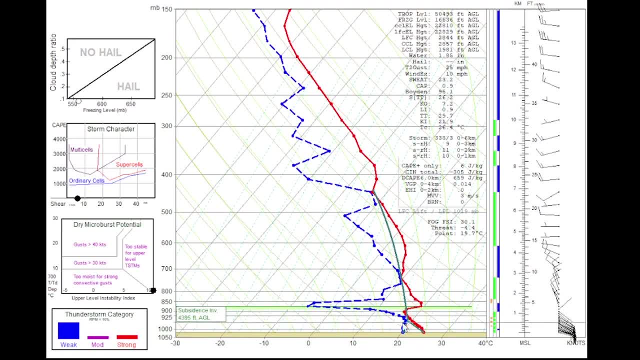 like that. you know that would cap any of that moisture on the surface and then, um, like i said, radio waves can travel through that a lot better, noise can travel through that a lot better, so you'll get a lot further distance on radios. another thing is low level wind shear do we have? 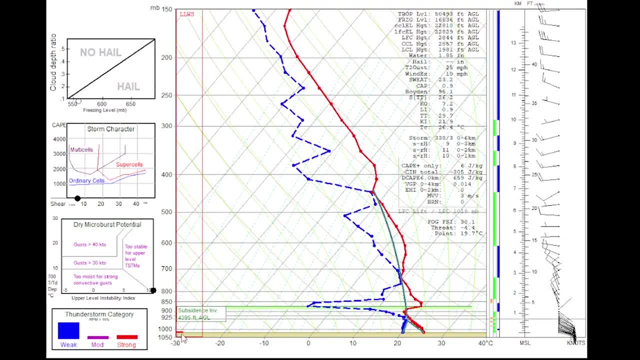 any? no, there's nothing, actually very that's. the surface might be a little bit of low-level wind sheer, but nothing significant on this chart. now the cape on this one. we are pulling six jewels. we don't even have any, really any energy in the air here, so we're going to pull home the. 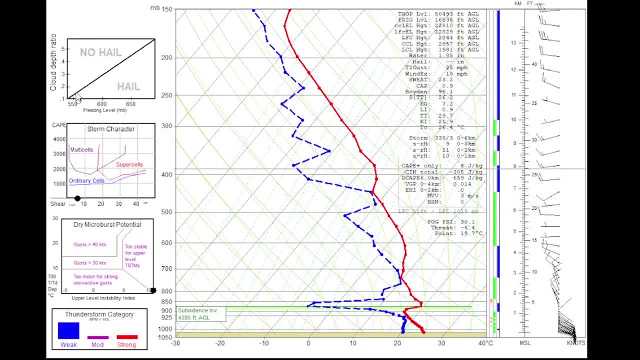 the in that system, so in this atmosphere. so we really don't have to worry about all that, but if we do, we gave severe weather. um, i'll start keeping an eye on that. maybe i'll do a video on that. uh, we'll pull this program and we'll start comparing it to real-time data. what's out there? 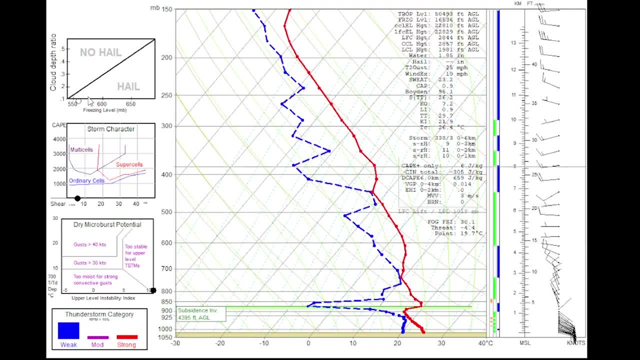 and then, uh, start pulling some of these values and see how accurate this, this scooty, really is all right. so relative humidity should put a line somewhere. just puts it over here. now let's go. uh, one other thing we can do is close that out. go to display soaring data. 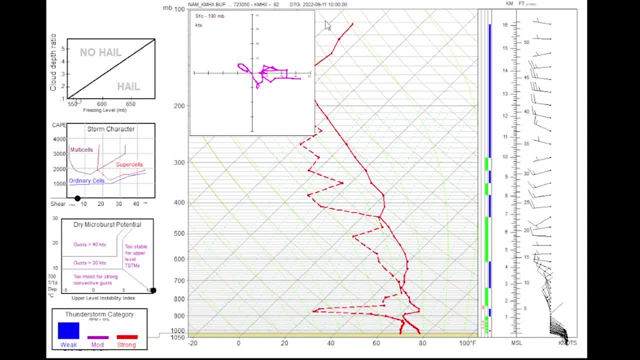 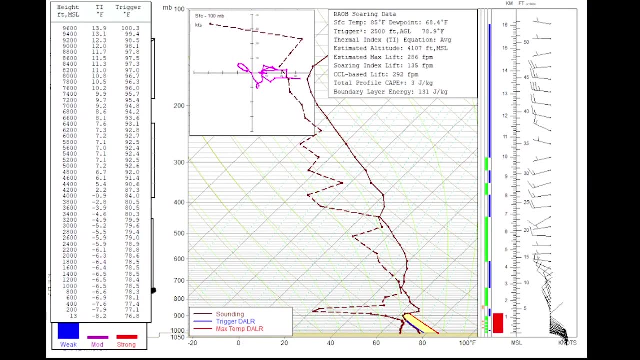 whatever our forecast max temperature is for the station. um, i'm not sure what that was. this is about 76.8 degrees. let's go. let's go 85, then we can calculate. now, if we close that out, we can when we put our mouse over this. uh. 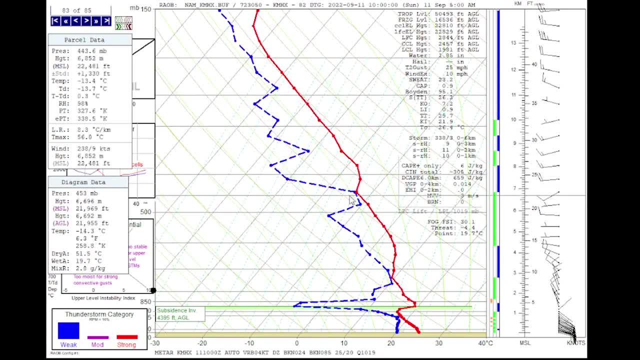 chart we can see all our values to the left. so our pressure height, mean sea level, temperature dew point, relative humidity, so we're going to how high we are. so now, when you see these things spread apart like that, you got a. you got a substance aversion in place. 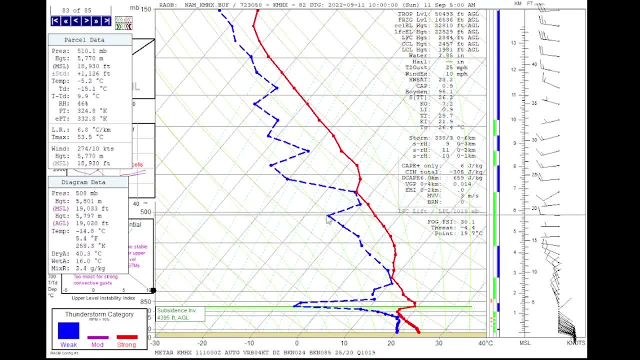 but you got a dry layer right above that. anytime they start spreading out, you can count them as just dry layers. now, when they're close together, then that's where you got moisture. um, do clouds again? we can see the clouds at that layer, clouds up at this layer and then 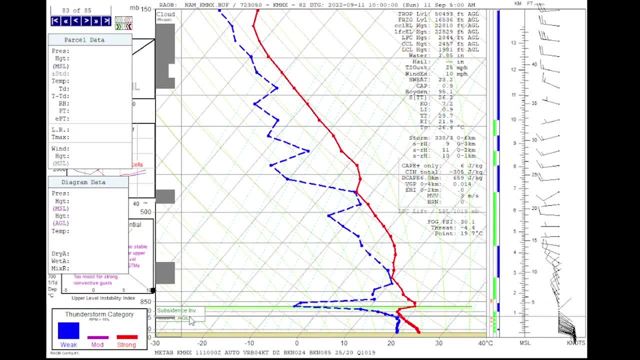 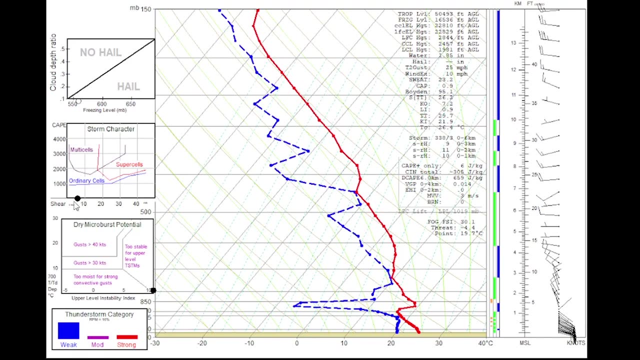 clouds at the lower levels. so then the substance inversion we have. we do got clouds at that layer too, um, being capped off by that inversion. but you, we can make our way through all of that and then we can see. wait for the next layer. all right, frontal layer. i don't have that option just yet. i didn't purchase that one. let's go back. 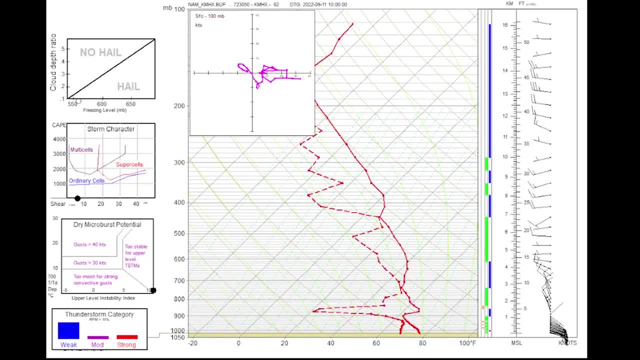 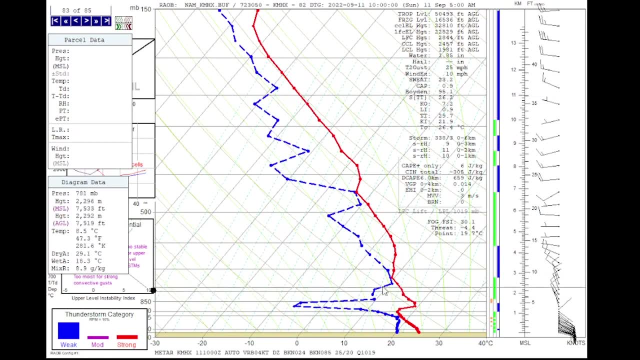 not what i wanted. all right, so we can follow these up. you can actually, with this program, you can- i think you can- forecast, I think you can analyze what you want. I thought you could. you can move these. I know on one part of this, I don't use this too often, but you get back into 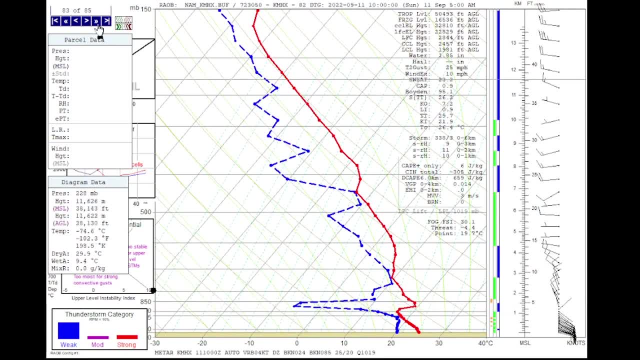 this thing again. you can actually move these temperatures and dew points, maybe with the current scooty. let's go. uh, let's go, pull the latest one open sounding. I got screens you. you can't see or you can see is the base screen, but I'm going back into the list and pull in the latest sounding. let's go to the. 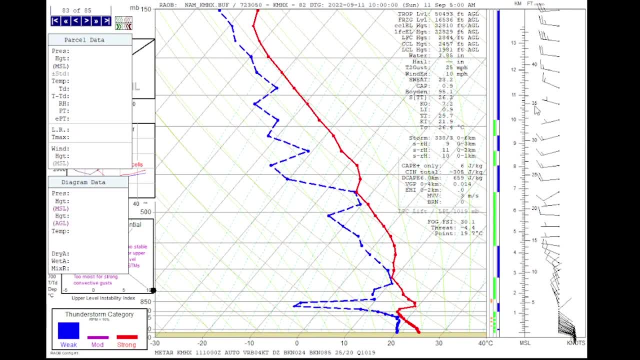 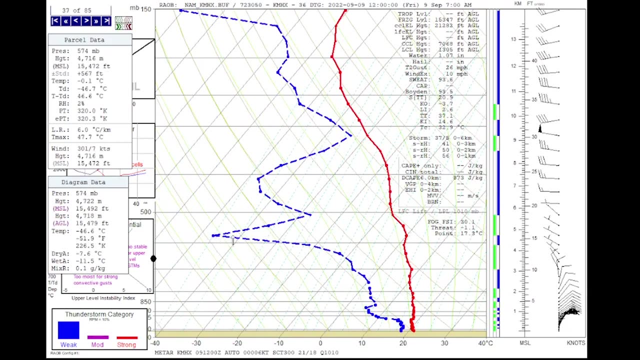 ninth, 12 Z would be the one, probably the 10th, at 0 Z, but we're gonna go good night at 12 o'clock of Z on the night, okay. so now I can actually move these and say, okay, if I do point increases at this layer, then we can say what happens. we change all of. 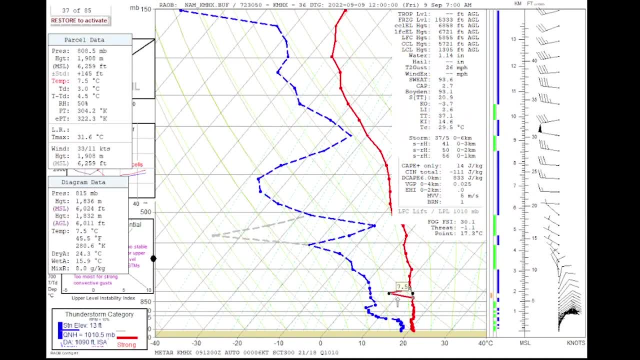 our values and give us a what if on temperature decreased. so when we talk about an air parcel, subsiding, compressing, getting warmer, then we can say: okay, the mid-level temperature that air should increase, you know, by four degrees, so we can increase, increase this, and then we're going to, we're going to increase the temperature that air should. 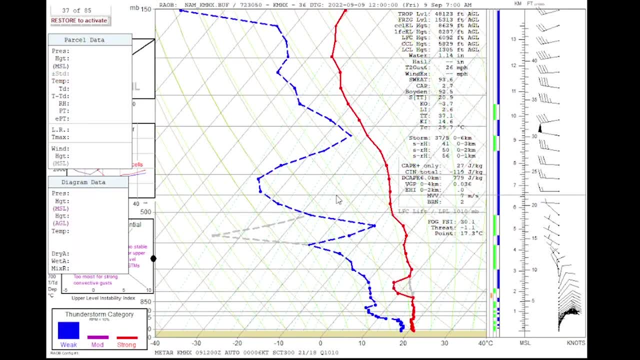 increase, so we can increase, increase this, and then we can try to determine how this air mass is going to be modified and then what kind of readings we're going to get out of that. so not easy, not an easy task, but it is possible with this program- the mid layers, if you got a. 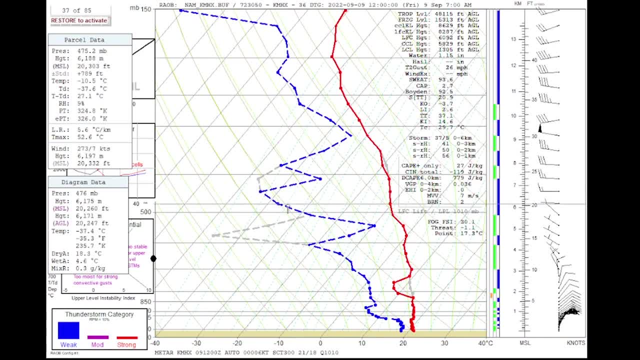 moist air advection and the mid layers and you say, okay, we know we're gonna go saturated at these levels. then we could pull this over to get them closer to the temperature with these dew points and then increase the dew point and then start showing different readings. capes only 27 joules. we'd actually have to. 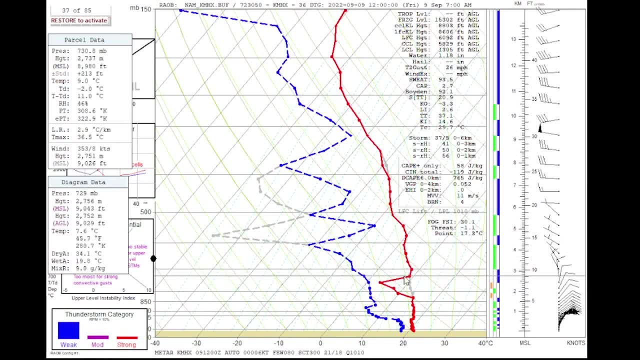 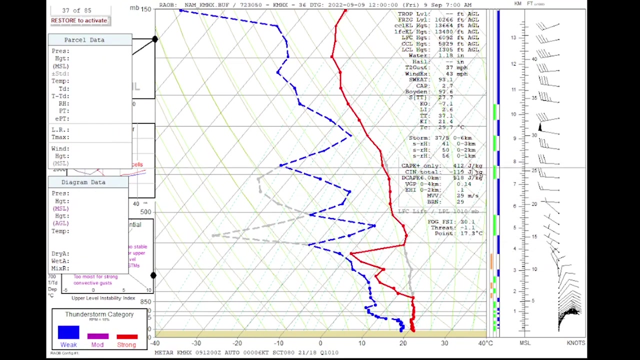 drop this way down to start increasing that. if I grab them, they're a little tough to get. you have to get each dot, so it's not working right now. there's one now. our cape went up to 412 from just for doing that, 484. you can see, obviously, when you get closer together, more saturation through. 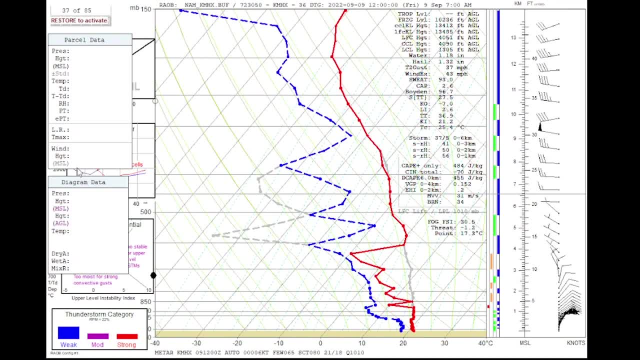 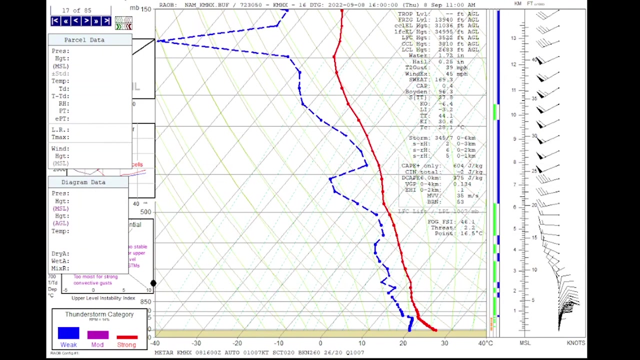 the upper levels, then you can, you know, have a higher energy level. all right, so restore, so you restore to activate. I'm not sure how to do that yet I'm going to open a sounding. okay, alright, so if we go, look at our LCL, CCL, carburetor icing, thermal low-level wind. 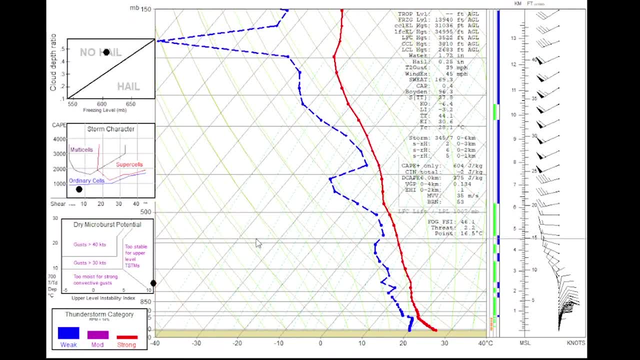 shear. you always gotta have a low-level wind shear to have a tornado, so keep an eye on that. now your wind speeds also like these wind speeds right here. they were coming out of the Northeast and then shifting over to the west and northwest, so they're backing with height, so that 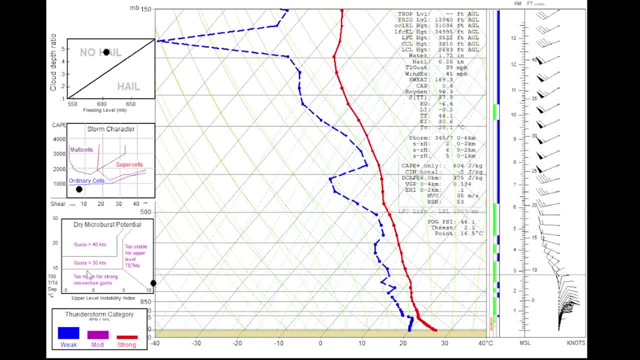 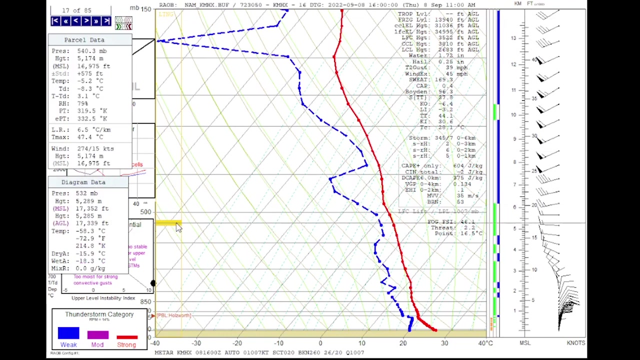 should indicate that there's cold air advection in the in the upper levels with the winds backing on height humidity- let's see mixing height off all the lightning okay. so possible area of lightning mean state level 16 with above ground level. here we got 17,000 feet, so it's our freezing level 13, 9, so we can definitely move. our load goes over out here. we may have to bite off another Wardle down to 45 grams. so we had another light and we just get to no wind now and that means the new decking is closed because it is 45, 7 Sy pikos again on the coast. the wind does not bother on any of it and you brandney. so every single. 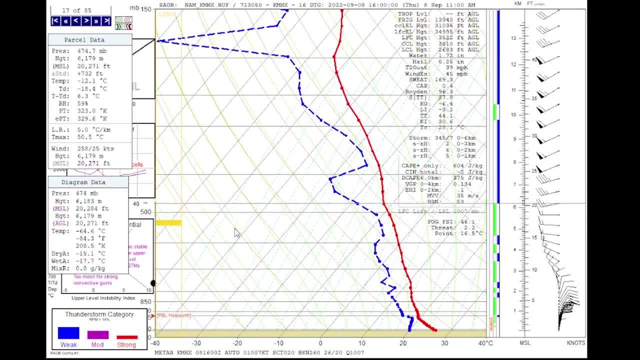 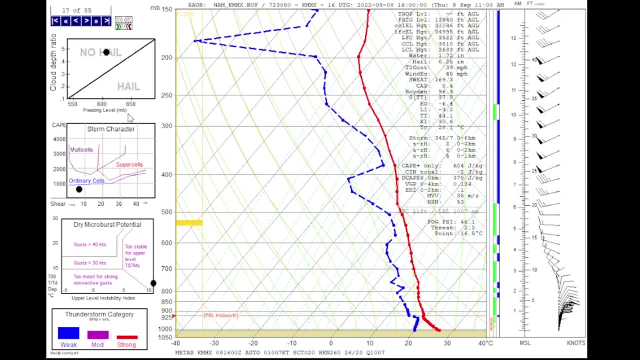 So we can definitely have some hail causing lightning. 17,000 feet Alright display for severe weather. That says Le Mans. Let me see what we've got. We can go. winter weather, fire tropical Photograph. Let me pull up a photograph real quick. 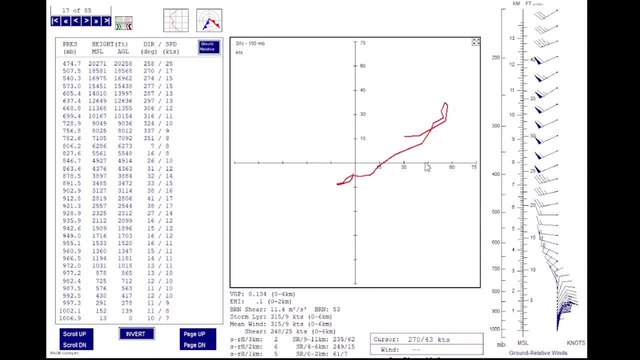 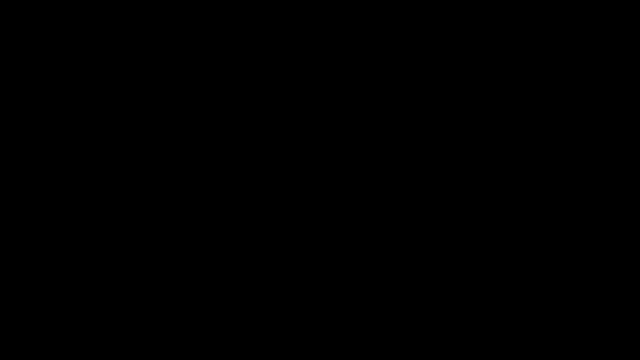 Alright, so we're looking for a nice curve on this photograph. This thing's kind of all over the place, so I wouldn't expect a whole lot to happen here. We'll just find a scooty. Oh, I just closed everything out. 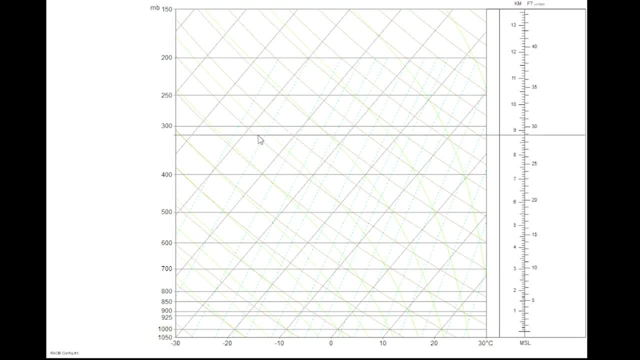 Okay, Alright, so I closed everything out. I just hit download again, so I've got it downloaded to every station across the United States. But I'm going to go ahead and end the video here. I'm going to say thanks for watching. 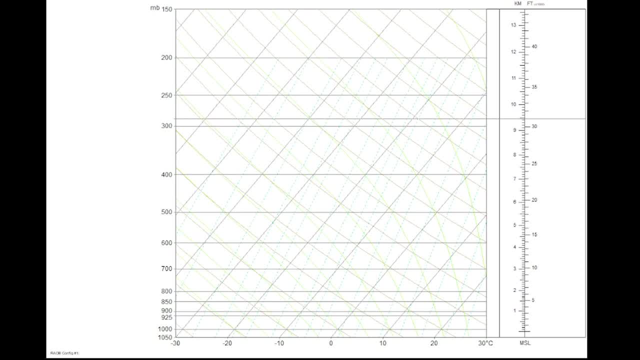 If you learned something, hit the thumbs up. And the next video we're going to be covering upper air analysis. So we're going to get into some upper air charts and how to read those And do some just some upper level, just reading upper level charts and telling what's happening in the upper atmosphere. 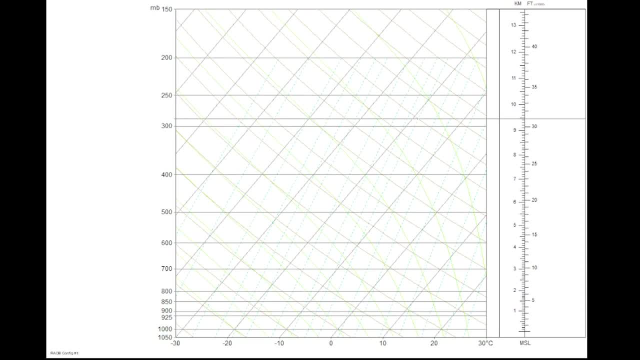 So, like I said, if you like what you see, hit the thumbs up and subscribe, Visit my website, meteorology101.com. And thanks for watching.